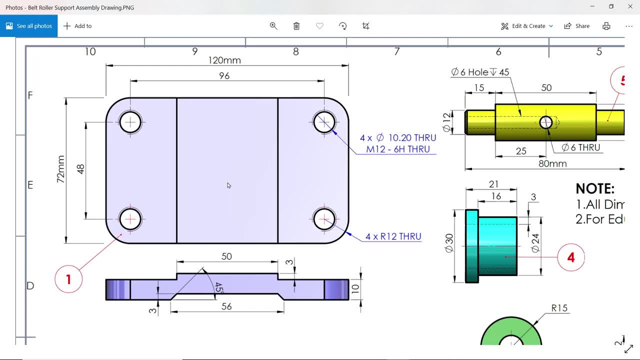 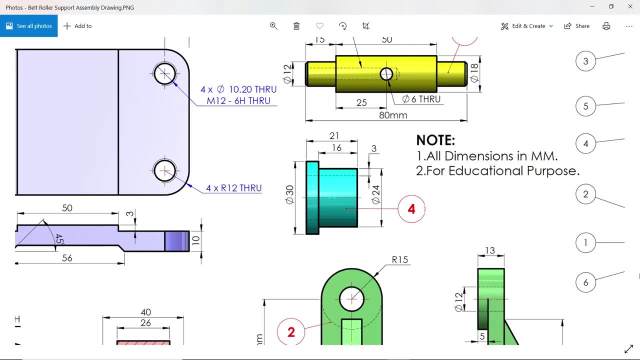 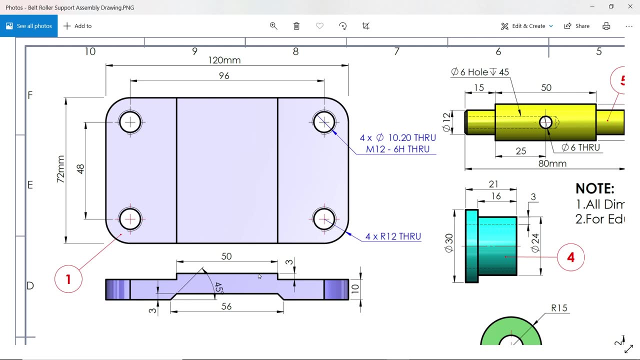 The first part of belt roller support is base. If you check in table all the things are written: base bracket, roller shaft. Now the size of base is 120 by 72 and thickness here 10 mm. Then there is one more surface solid parts feature, going to add 50 mm, 3 mm thick. 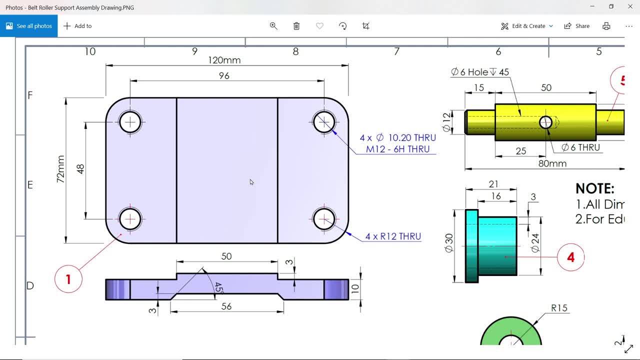 Then corner radius, you will see 12 mm 4 corner And in this corner there is a M12 tabbed hole. This is tabbed hole and we will use hole wizard tool to kill it. See the center distance, but actually it is located at the center point of this arc. 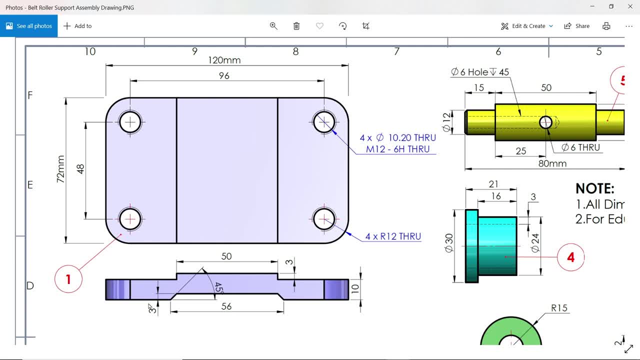 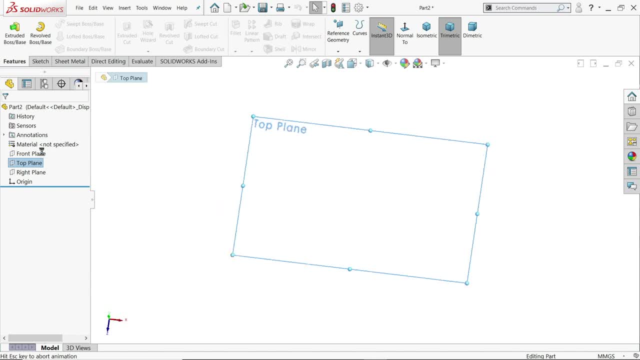 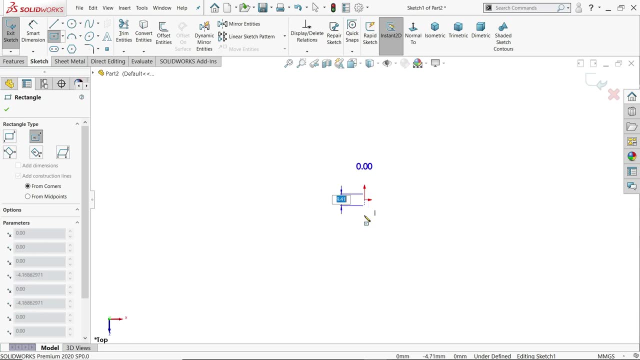 Now at the bottom there is one cutout: 56 mm, 3 mm height and 45 degree. So let's make the first part. So I will choose here: top plane sketch. Now go to sketch and activate center rectangle. Now This one. 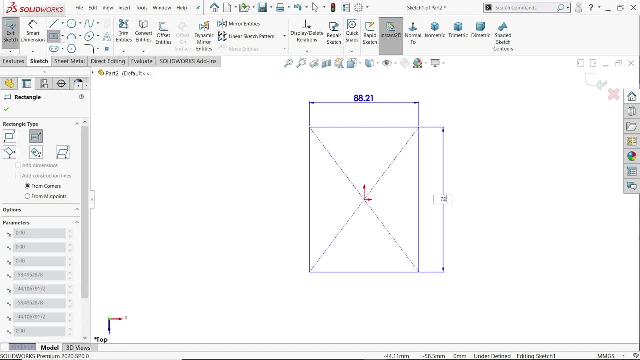 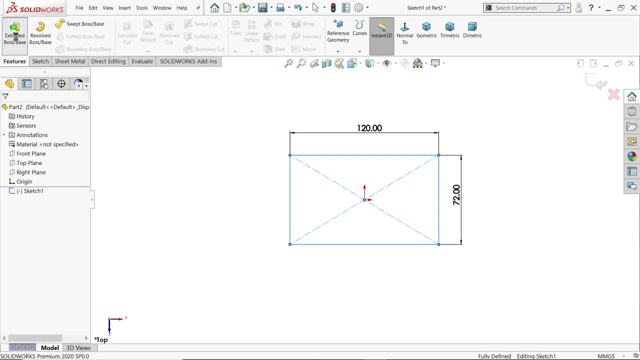 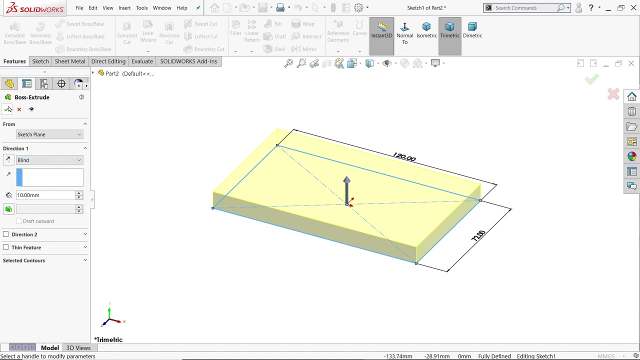 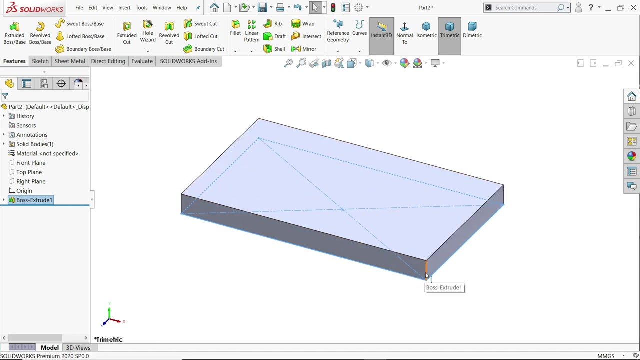 72, tap 120. enter Now here. go to feature and choose extruded boss base. See Now. keep end condition: blind: 10 mm thickness. say yes. Now, if I am going to choose corner, you will get two options: fillet or chamfer. 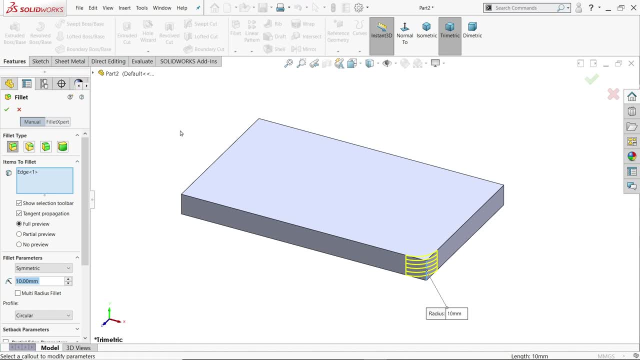 But here I am going to activate from here: Clear, Constant size fillet, 10 radius. If I am going to choose any one edge, you will see two options here. First one: It will automatically select all the edges, no need to choose separately. 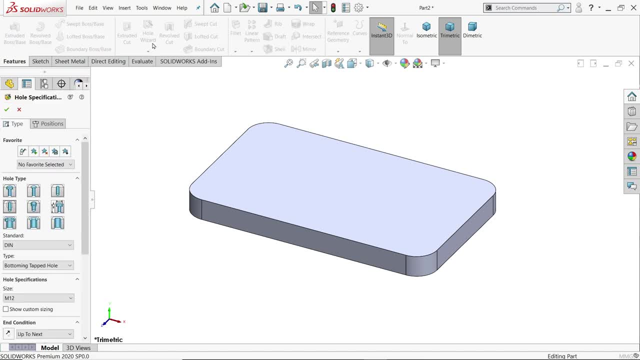 Say ok. Now I am going to choose hole wizard Now here, tabbed hole or straight tap option here: DIN standard bottoming. tabbed hole means Hole. Tapped hole is straight hole, no need to make any taper. And this is M12.. 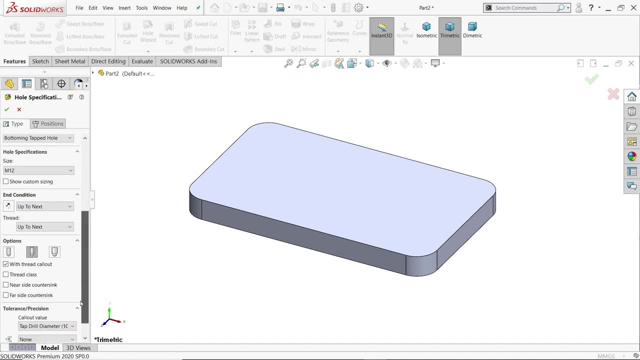 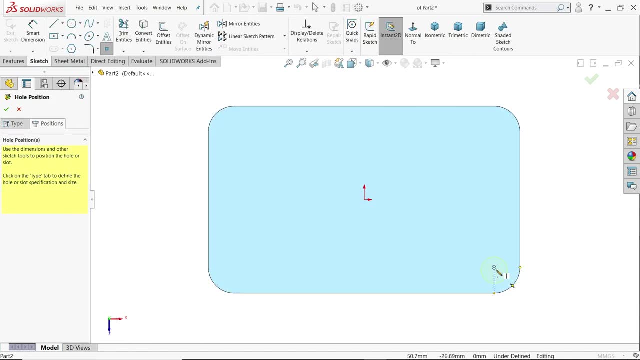 And condition: keep to next Position. I will choose this one Now. move your cursor to edge and you will find center point. Ok, And this is M12.. And condition: keep to next Postion. I will choose this one Now. move your cursor to edge and you will find center point. 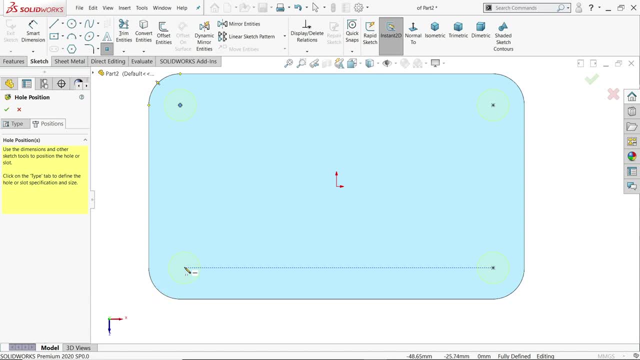 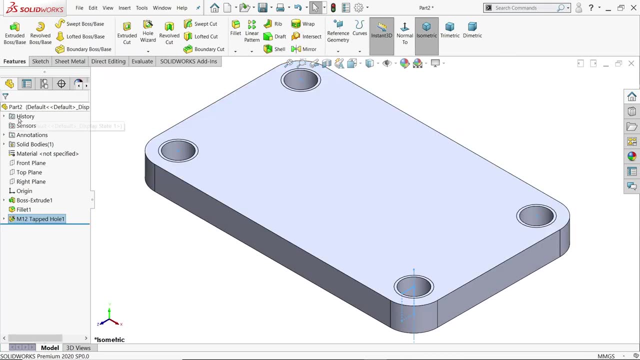 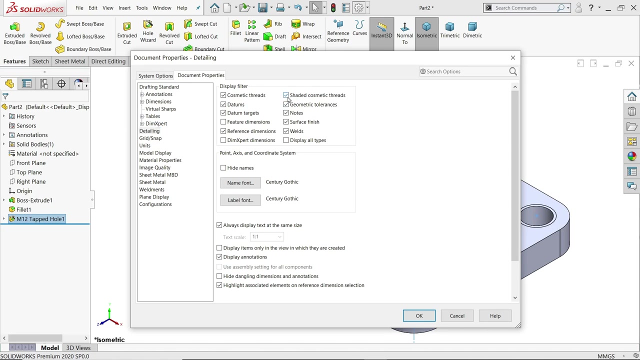 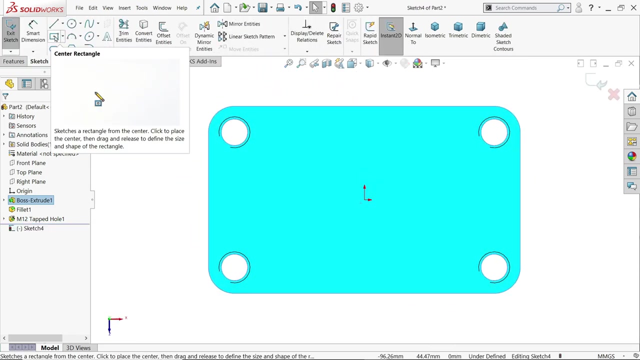 Ok, Now I am going to choose to center point And this is M12.. now skip key to out. check isometric view. say yes. now click options, documents, property detailing and check the shaded cosmetic thread. say yes, you will see the sketch again. I'll activate Center rectangle because this is located at okay. 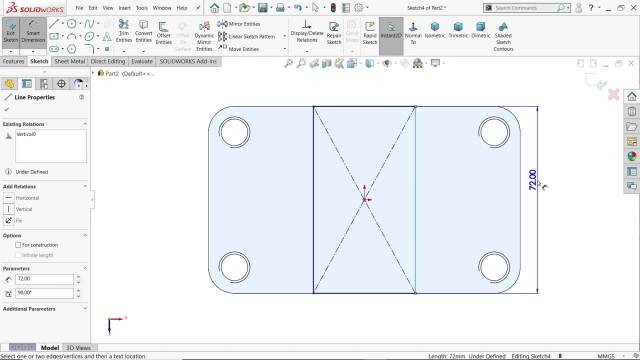 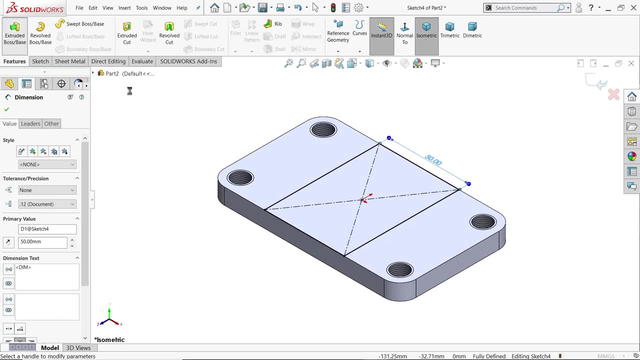 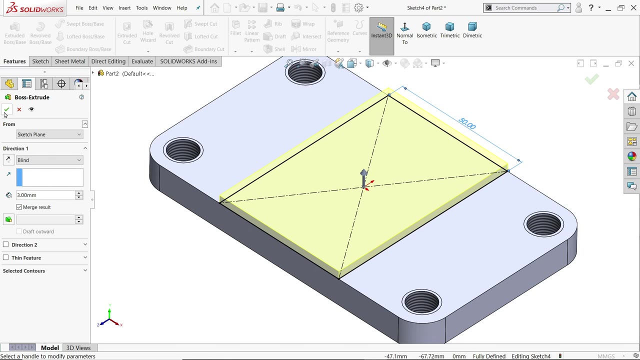 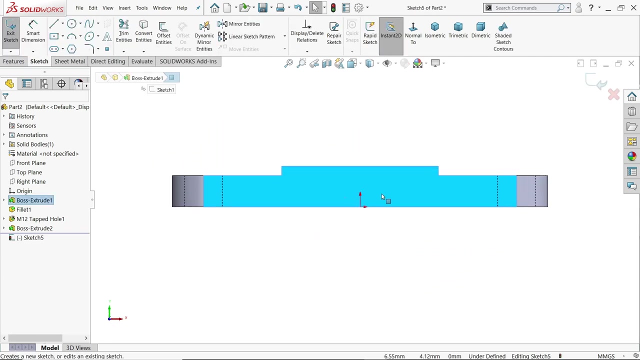 activate a smart dimension and we have to know, we have to define the horizontal length. it is 50 millimeter. feature and activate extruded boss base feature. keep here and condition blind and depth is 3 millimeter. say yes, look, select this face is sketch line. 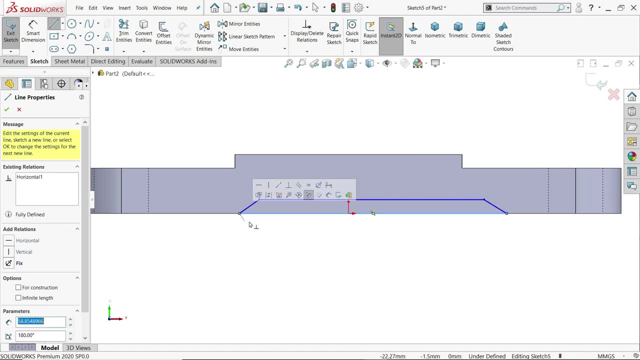 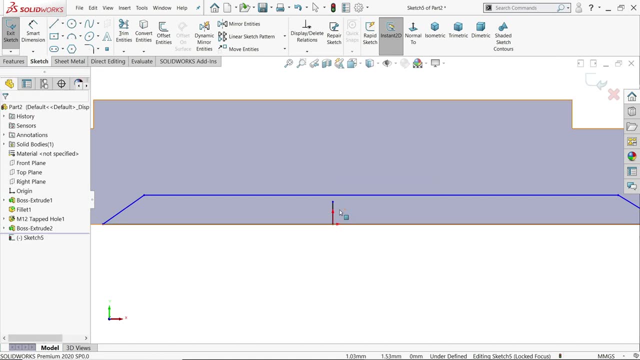 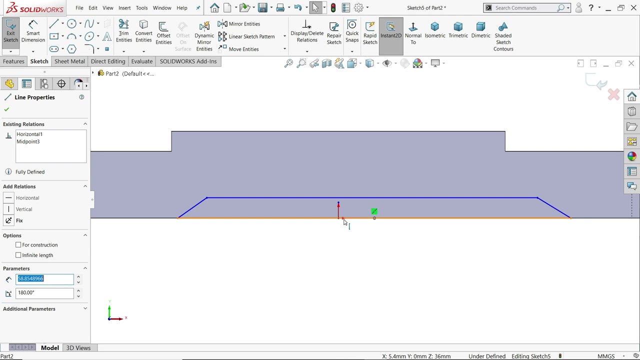 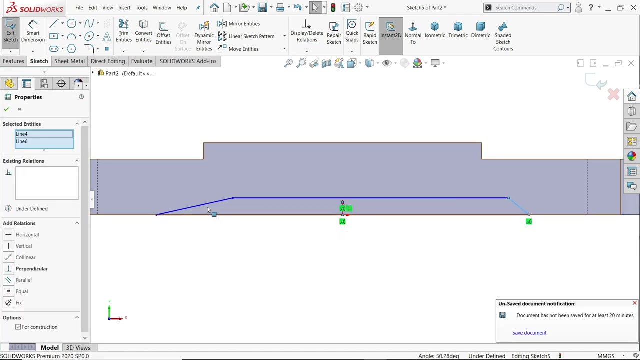 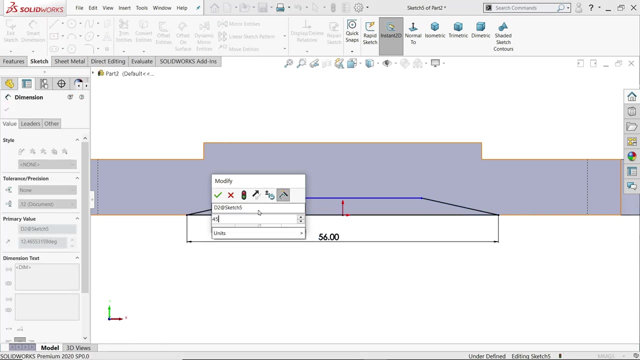 connect again. I'm going to draw one line, construction line. this is the center of this point. hold, shift key Center and origin point coincide. okay, now let me select the circle line and choose these two lines and make relations symmetric. activate smart dimension 56. let's make angle 45 degree and the depth is three millimeter. now see. 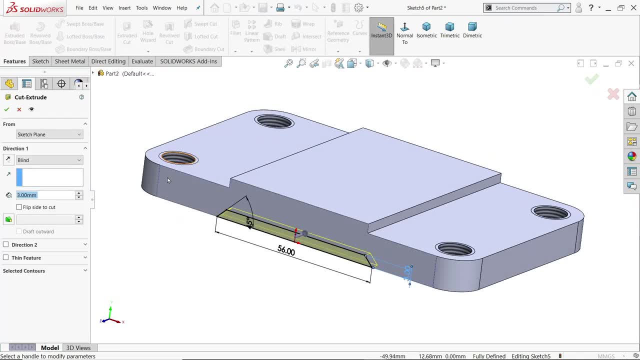 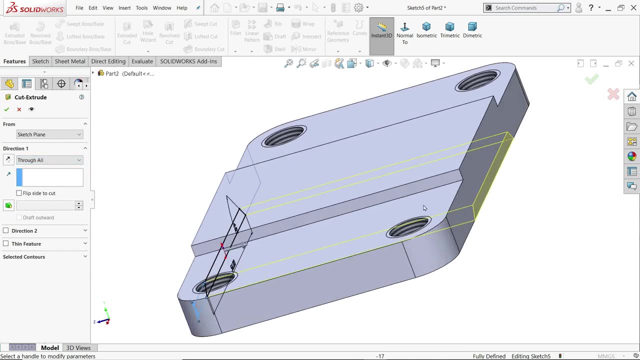 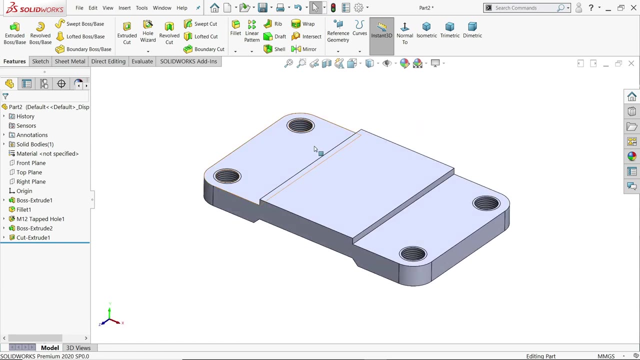 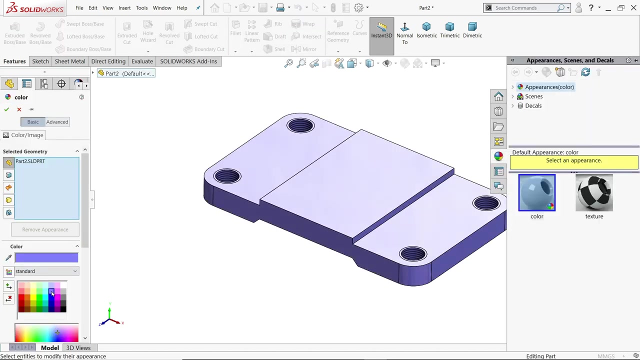 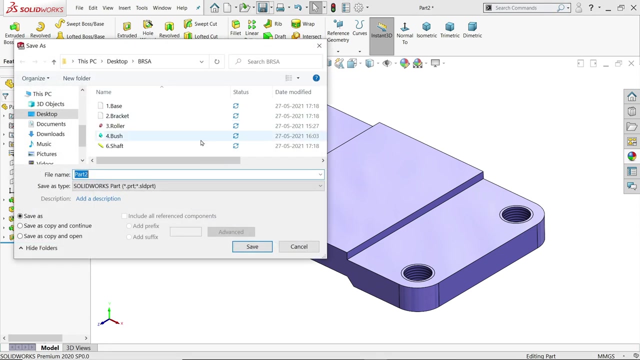 go to feature and activate extruded cut tool. keep end condition blind and depth, no less. choose through all see is going to cut up to this end. that's it. i'll add some appearance to this. okay, now let's save this one new folder. belt roller support assembly. 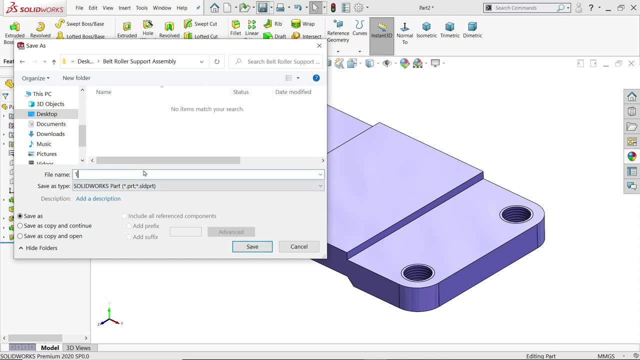 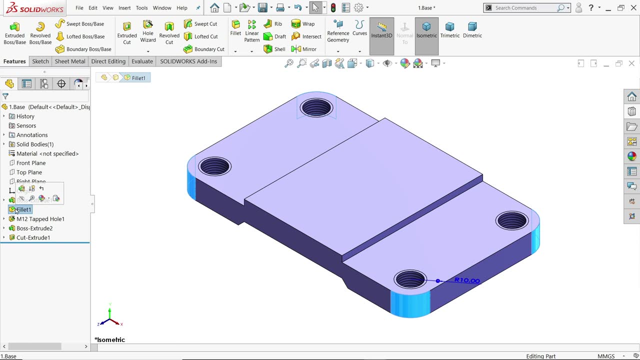 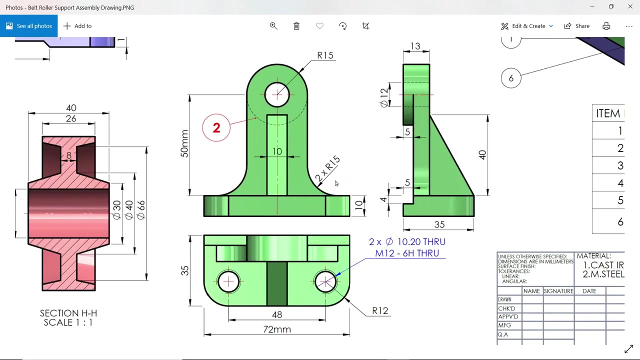 open part one. this is base now here. we forget to rectify this thing. fill it. you will see here. this is 12 millimeter now save. let's go to new part now here. the next part is side support or bracket bottom. we will see 35 by 72. we will use this one then. 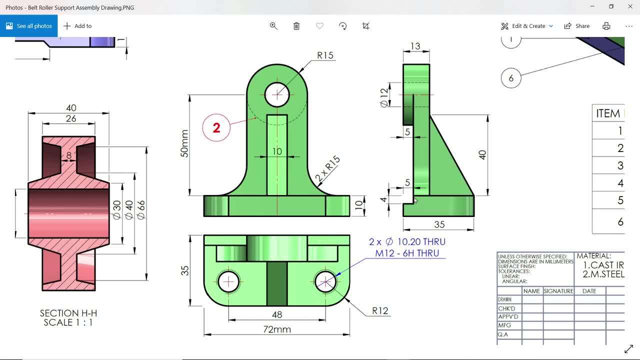 thickness is 10 millimeter. then from back side there is a flange. you will see this one r15, 50 millimeter from here, and this thickness, you will see 30, 13 minus 5 is 8 millimeter, and this is 5 millimeter away from this outer surface. 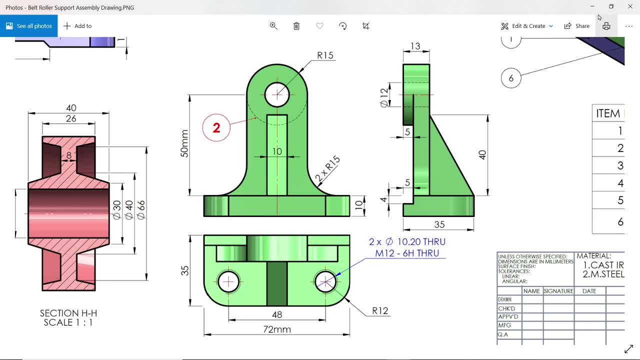 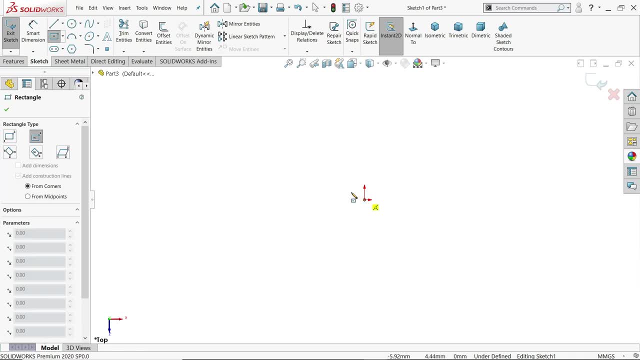 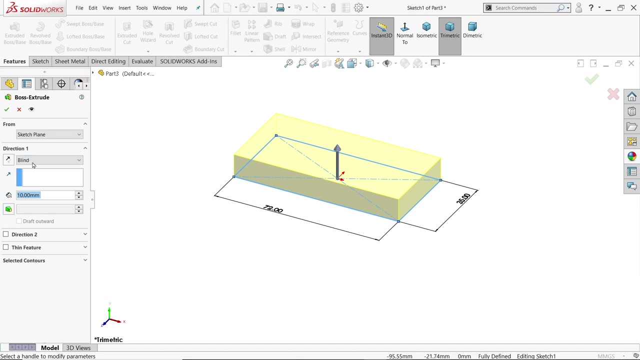 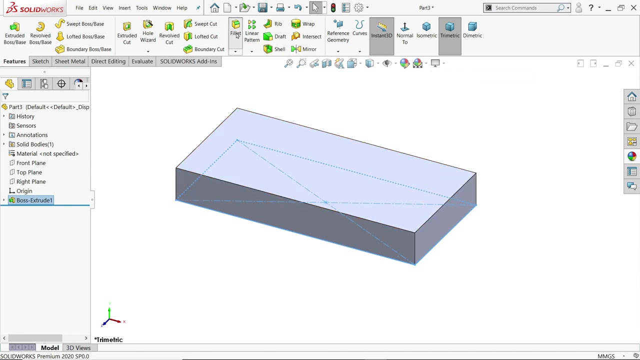 then later we will cut this surface: 5 millimeter. depth, 4 millimeter top plane, activate center, rectangle 35, tap 72, enter. extrude now this depth, 10 millimeter, and condition blind. let's again fill it, if i am going to choose one edge, and this is 10 millimeter. 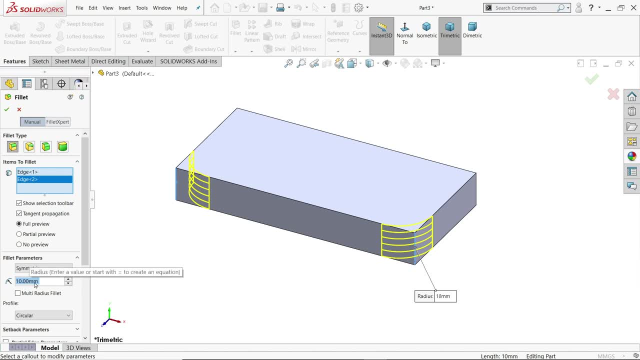 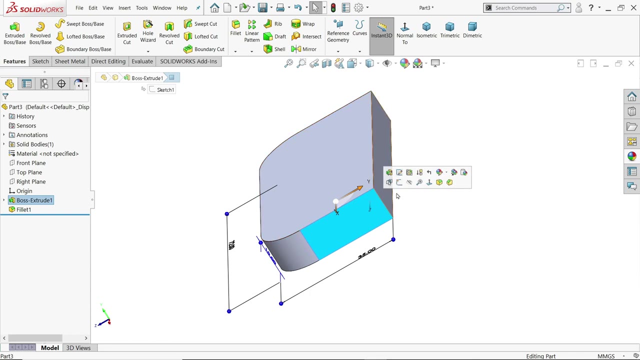 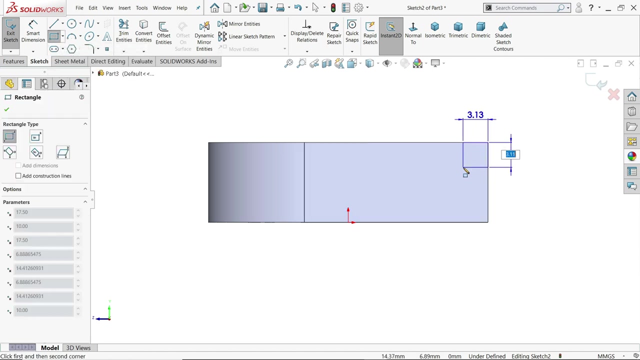 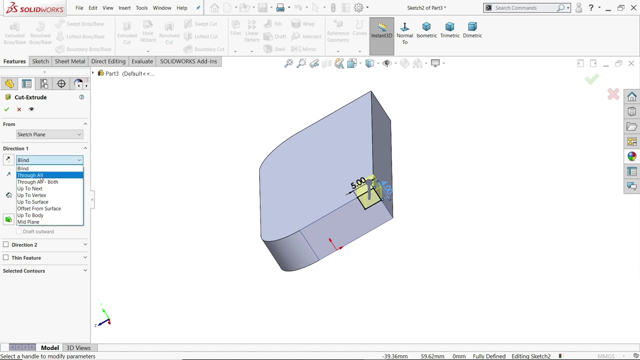 and condition blind. this radius actually 12 millimeter. okay, now from back surface. okay, we want to cut here 5 millimeter, so i'll choose sketch and activate center rectangle. now this length is 5 millimeter and this one is 4 millimeter. body log takes this every been Ihook. let's use water. 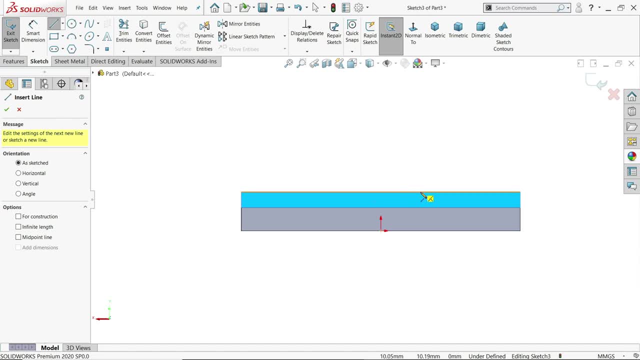 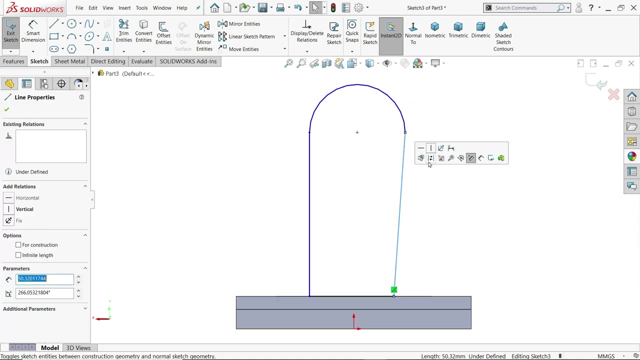 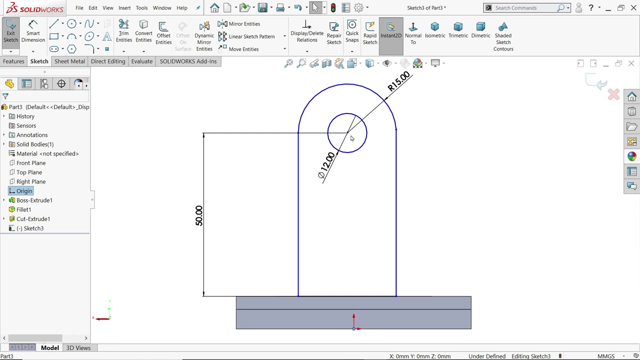 and we can move this flow to initialize theEmblem got that, we speak it in case. so back to image. finally, smooth tourism. so let's change god view as я. vertical activate circle and there is a 12 diameter circle, smart dimension: 50 now. distance from here to here is 50 millimeter. okay, one more: this origin point, hold shift key center. 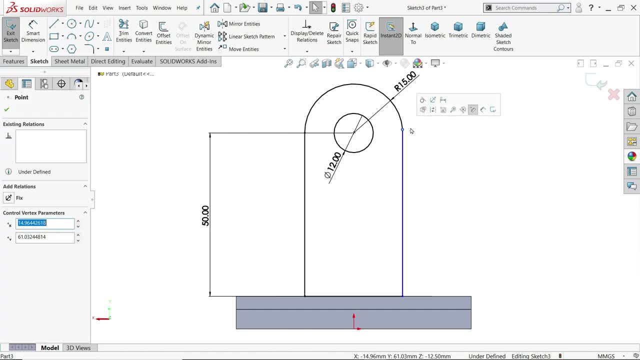 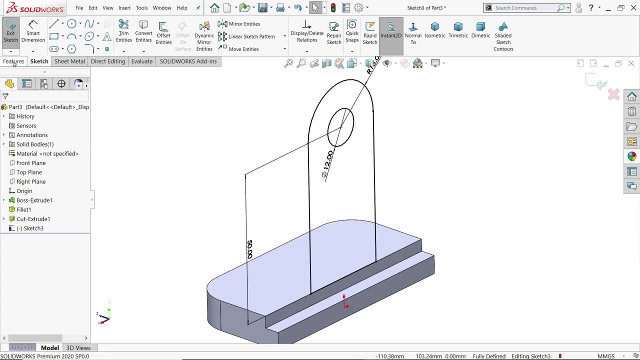 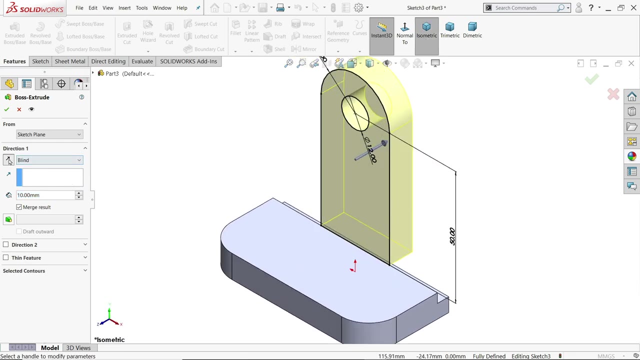 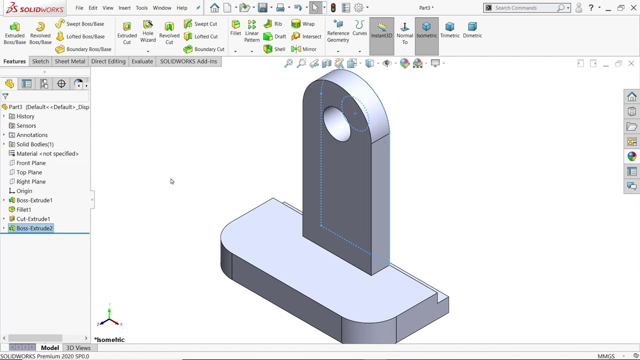 okay, this point is not tangent. now see, this is fully defined. a sketch activate excluded boss base feature. it is moving back side, reverse 8 millimeter. 13 minus 5 is 8 millimeter. okay, corner fillet is 15 millimeter. I am going to choose both. the end say okay, whole wizard. now here also tapped. 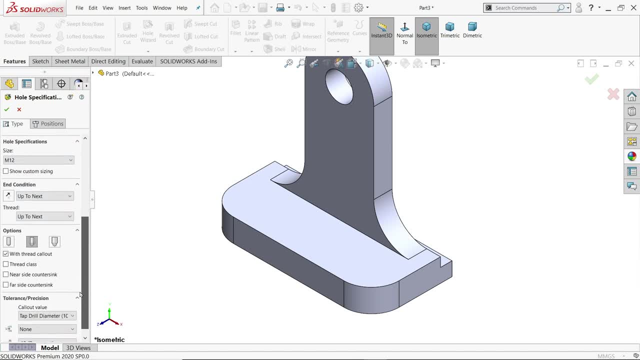 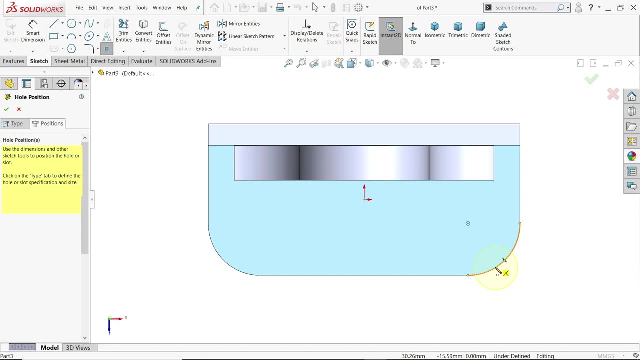 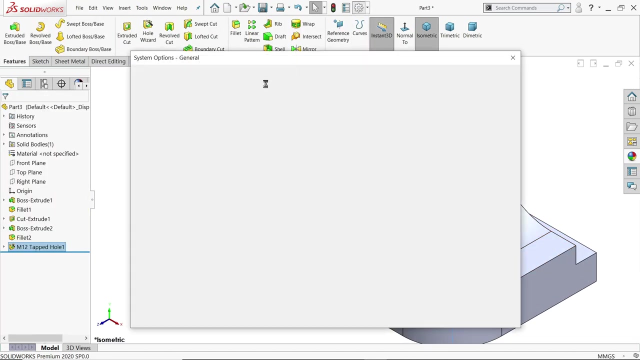 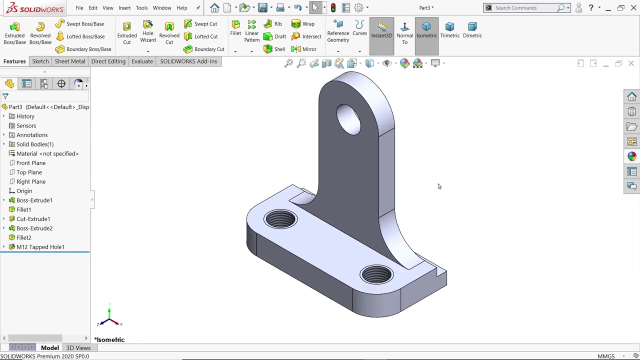 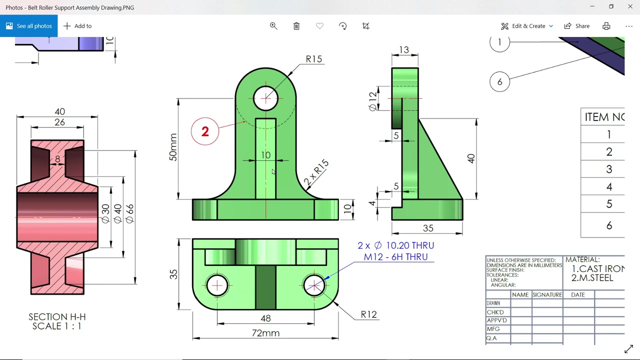 hold bottoming depth and 12 up to next with thread. call out position. select this one. keep cursor near here and you will find origin point or center point for this arc. escape key to out isometric view. say yes, options. document property detailing shaded cosmetic thread. that's it. now. here this threads everything applied. now this corner fillet also there is. 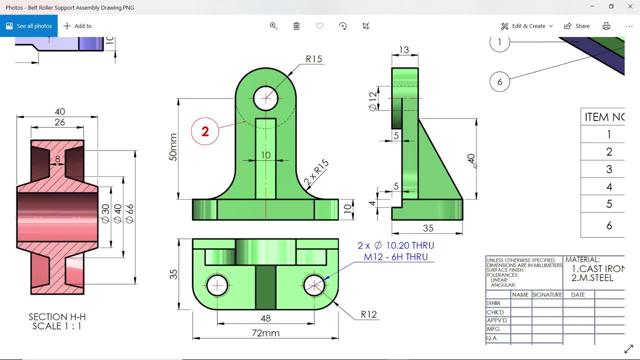 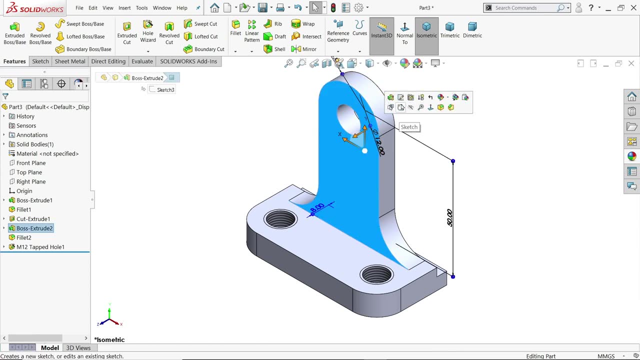 one rib 10 millimeter, 40 length. and here you will see these are 15, 30 diameter circle and extrude up to five millimeter. I'll select the space that face, its faith back face is catch circle and this diameter PCIN bars base and the distance it's five. 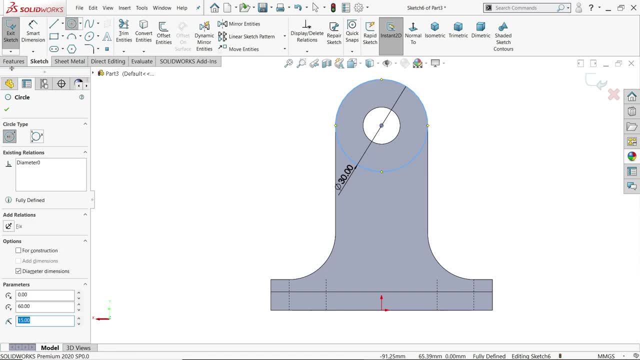 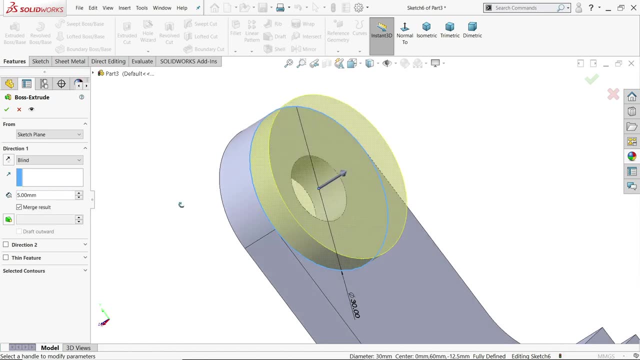 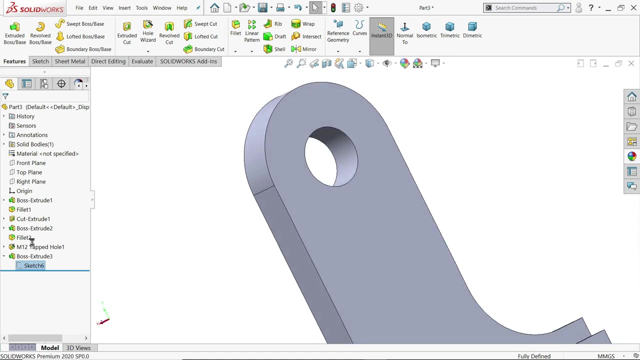 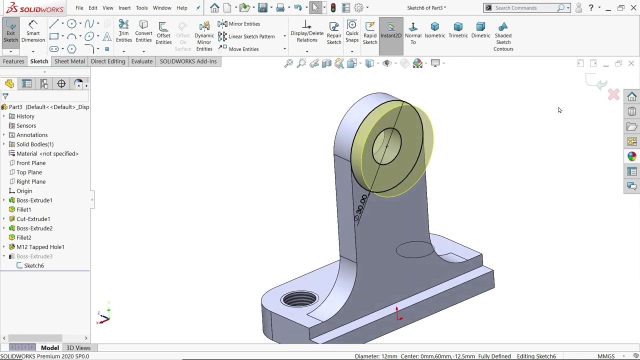 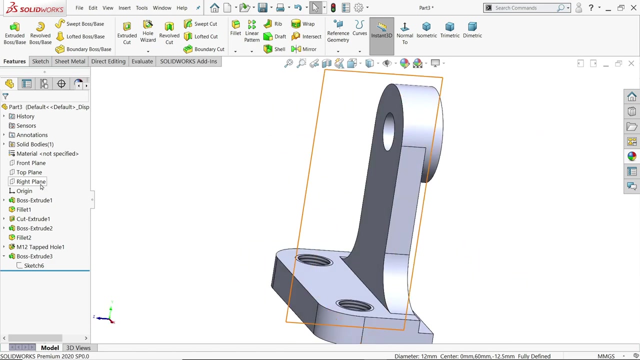 million and say, okay, now it is solid. so, of course, defined the found a a. no, got it. okay, got it, got it. we will do again. we will go to sketch, edit sketch now, click this circle inside circle, convert entities. okay, now, see the hole is created for rib. i'm going to choose right plane sketch now can. 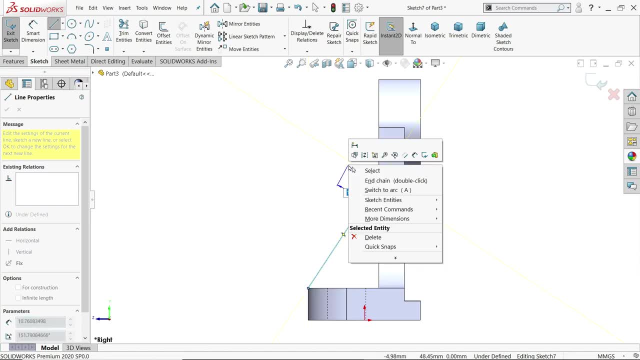 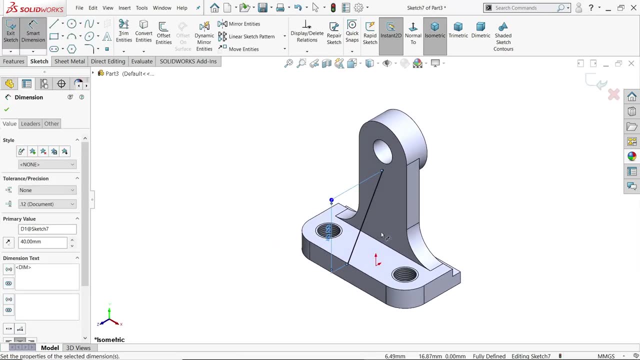 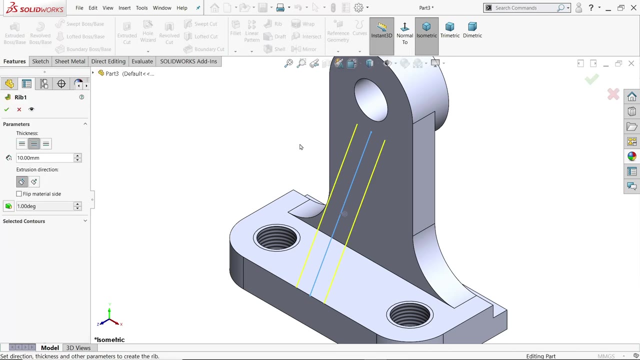 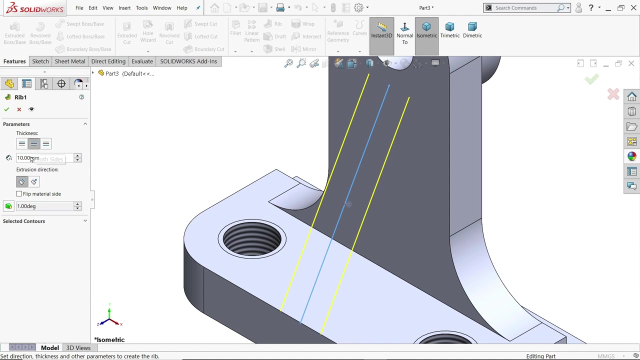 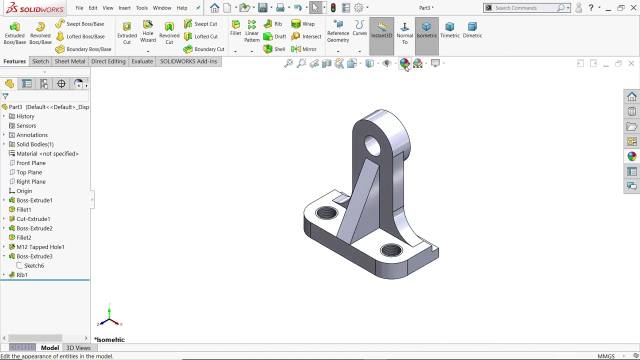 activate line tool and connect from somewhere here. activate the smart dimension and make the length 40 millimeter. exit and go to features. check here rib rib feature. see, you will see the arrow is going towards body thickness, both side 10 millimeter. say okay, look okay. 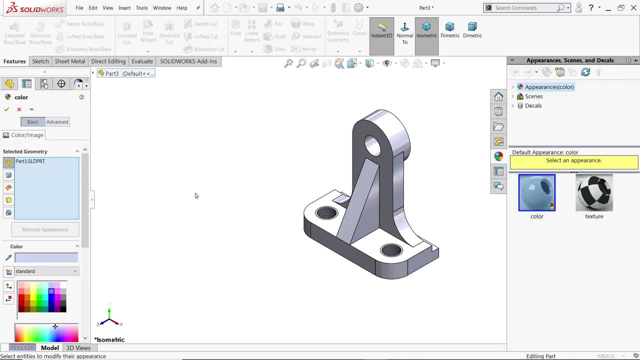 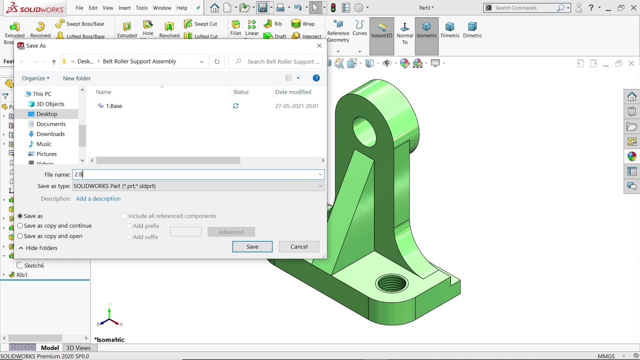 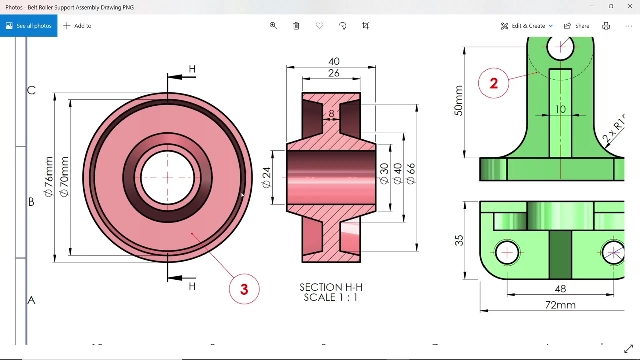 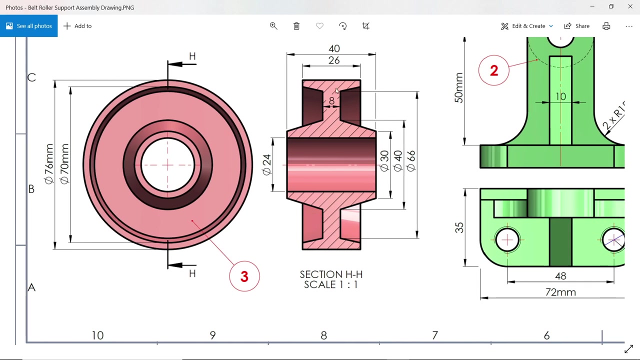 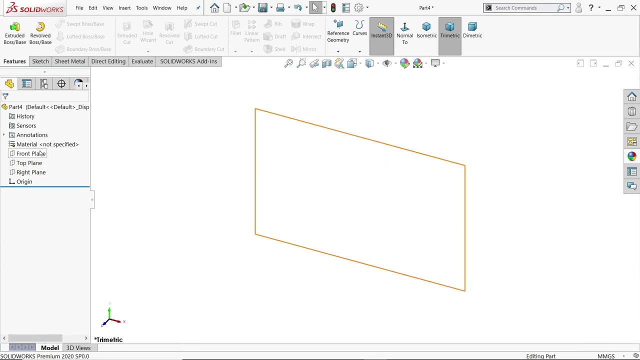 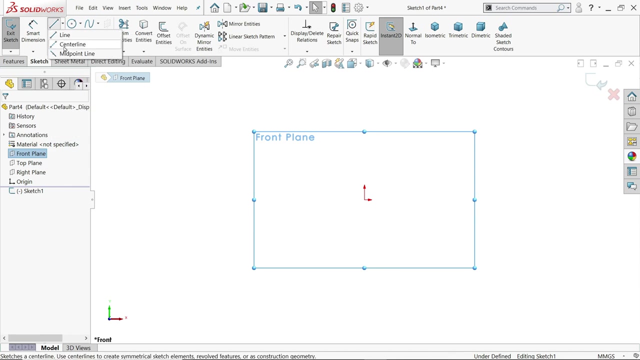 okay, now i'm going to activate this. okay, this one is sufficient. this is the part two bracket. now here, the third part is roller. what names we suggested for this roller? okay, okay, so '' okay, right here. okay, front plane is sketch. now, first let me make center line. okay, now activate line. 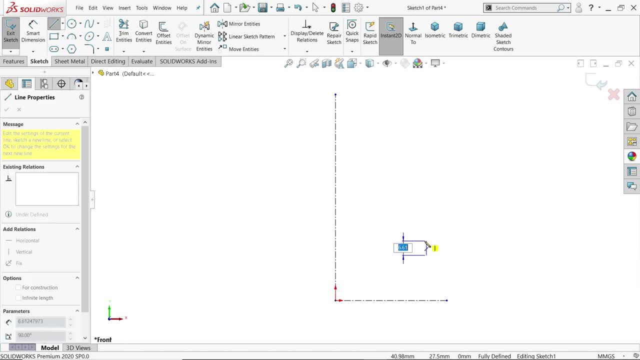 tool. now start from here. better to use dynamic mirror. select the line now. activate line tool. see, don't create any relation, otherwise it's difficult for us. okay, now deactivate again. activate line and connect. that's it. now it's time to define the dimensions. now this one, if you move. 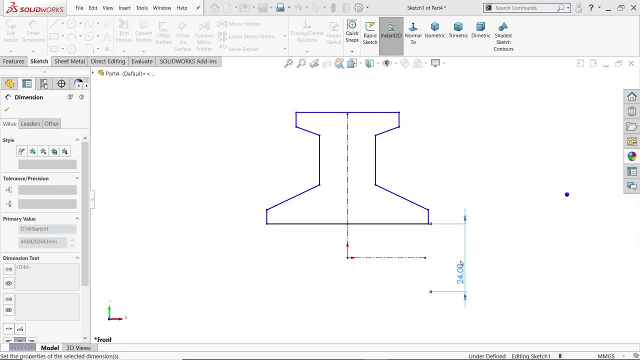 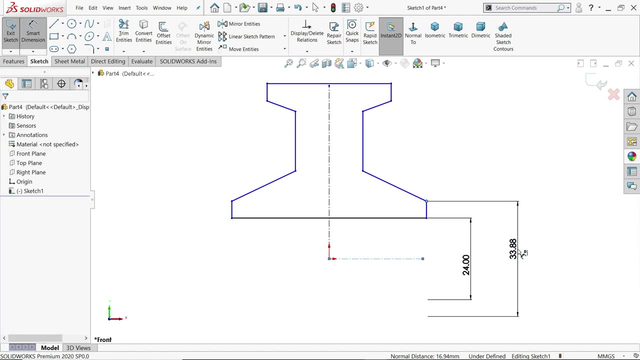 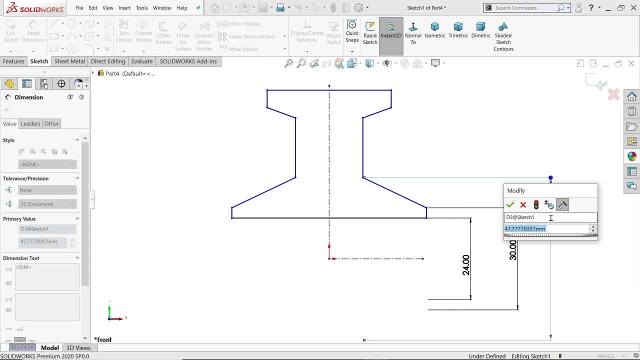 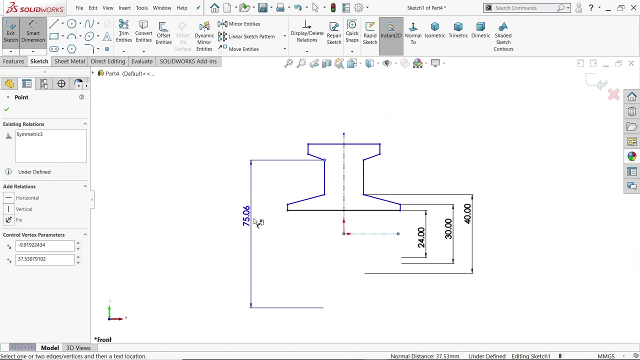 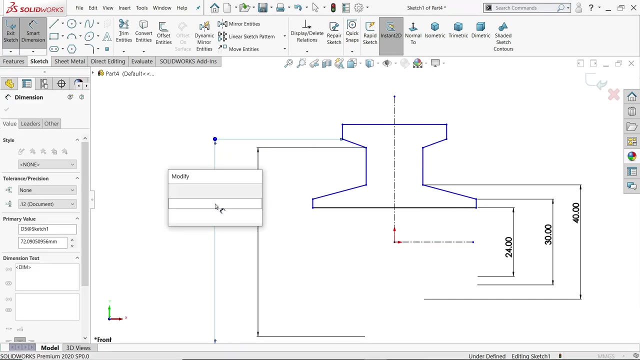 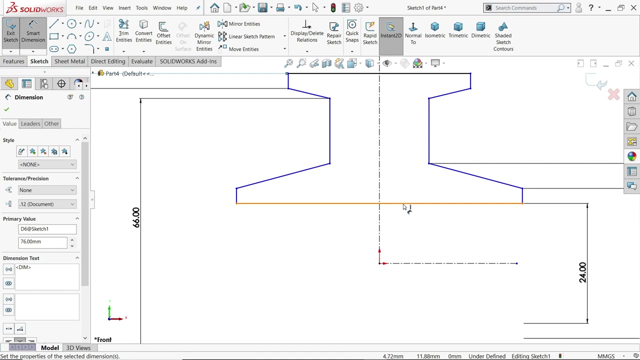 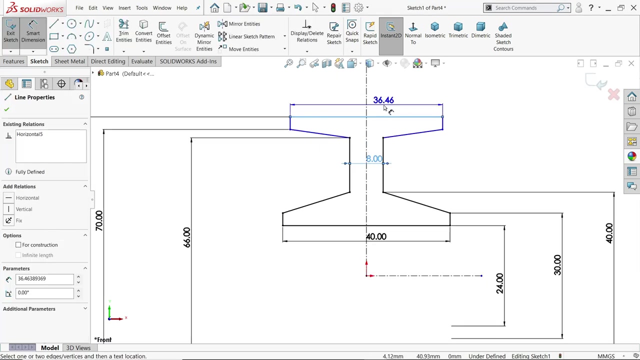 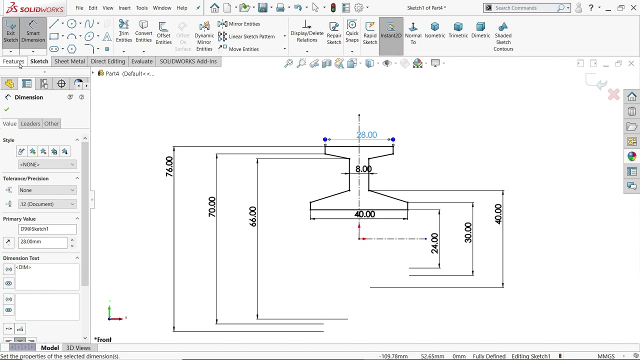 downward you will see diameter. so this is 24, the second point 30. now the third point 40. now this point 66, second last 70 and the last one is 76. shift 40. now let's make this distance 8 and the last one 28. now see, drawing is fully defined. we defined all the diameters. 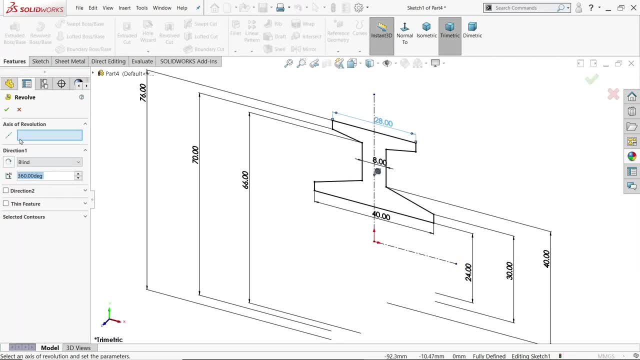 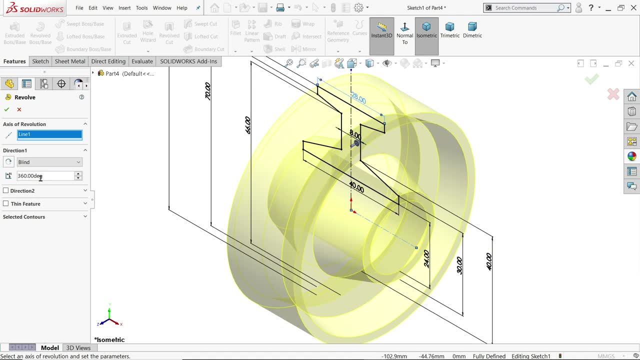 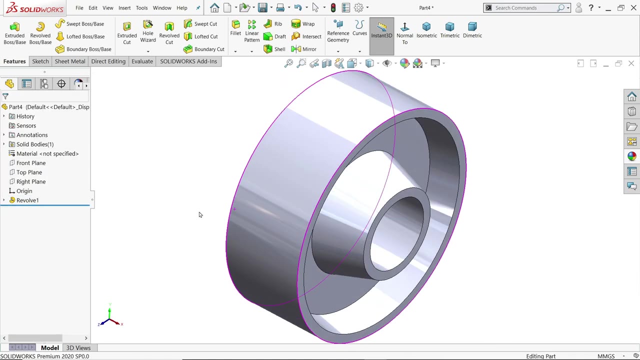 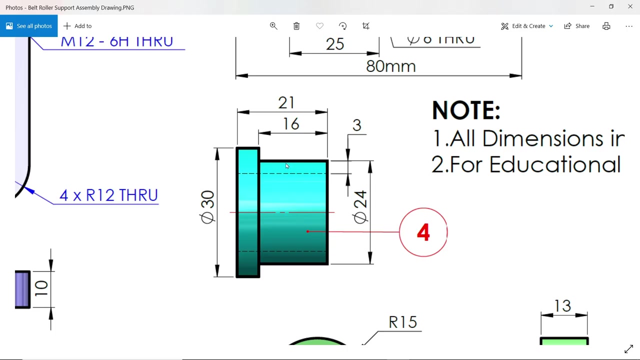 revolver boss base feature. axis of revolution. I'll choose this line. you will see the preview angle of degree or angle 360. now save this one. part three roller. now the part four is bush: outer diameter: 30, 24, 3 millimeter thick. here 16, 21. we will use revolve boss base tool front plane. 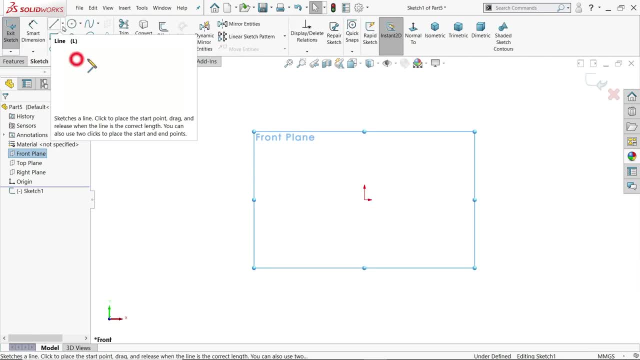 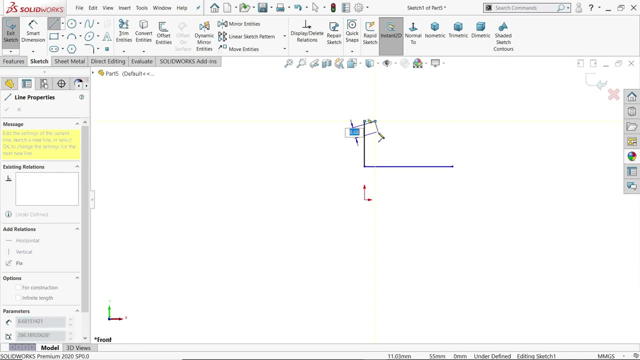 is sketch. now let's activate line tool. I'll start somewhere: front plane sketch. now let's activate line tool. I'll start somewhere front, from here, vertical. now make a construction line which help us to revolve a body in it can horizontal construction line hold shift key and make in one line horizontal. so it is for now this one and this one. 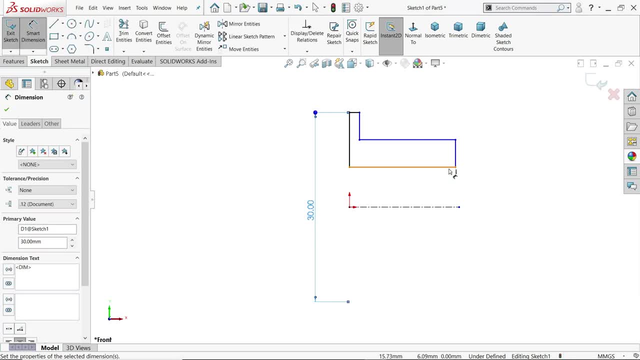 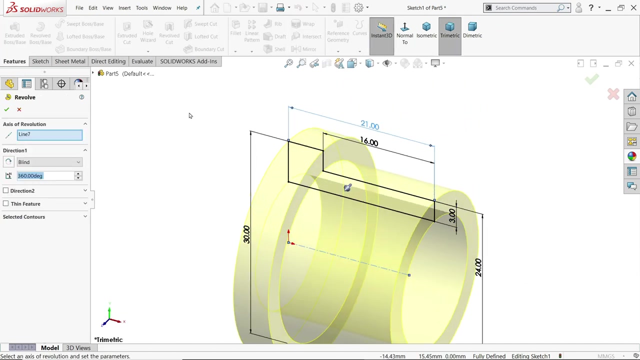 Now this one: 24, 3 millimeter. distance from here to here, 16 millimeter, and the distance from outer edge to outer edge 21 millimeter. Now go to feature and activate revolve boss base tool. see, it automatically took the line. 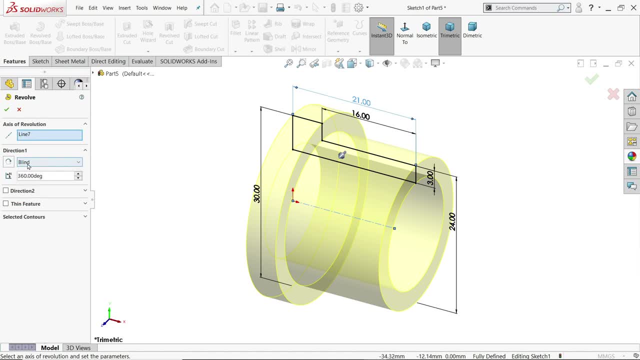 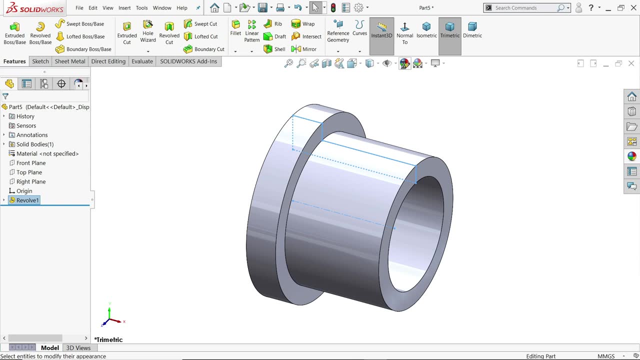 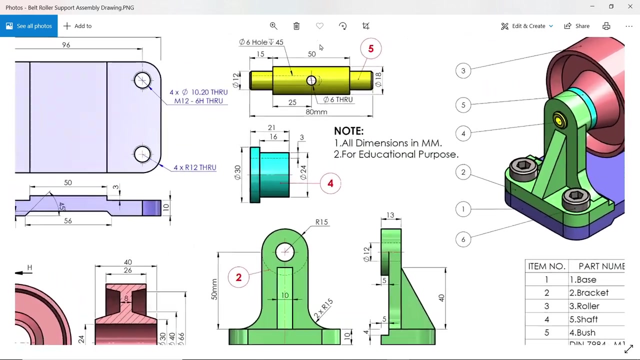 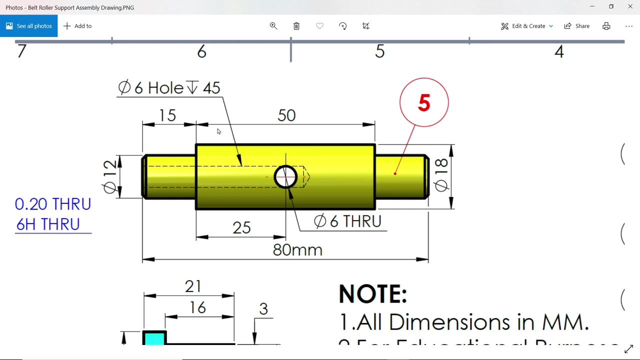 center line or axis of revolution and condition. we will keep blind and rotation 360 degree, say yes, okay, this is the part number 4, bush, Now here. Next part is shaft: 180 millimeter long, 50, 15, 15 the center diameter, 18, this one 12 diameter. 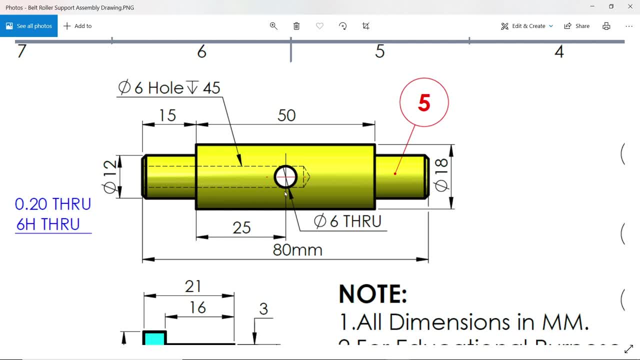 and there is one hole 24 millimeter, 25 millimeter from here to here at center, 6 millimeter throughout hole, and there is one more hole inside hole and this is actually. this is pin hole: 6 diameter, depth, 45 millimeter and corner chamfer is 1 millimeter. 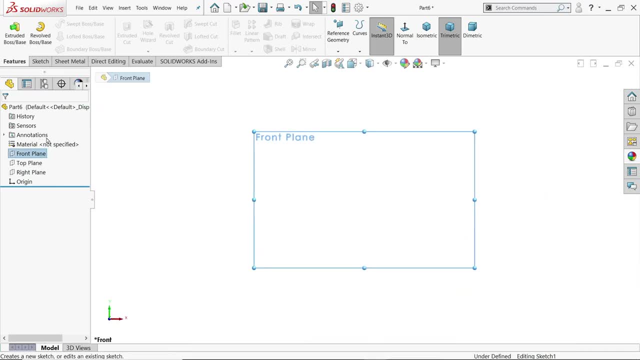 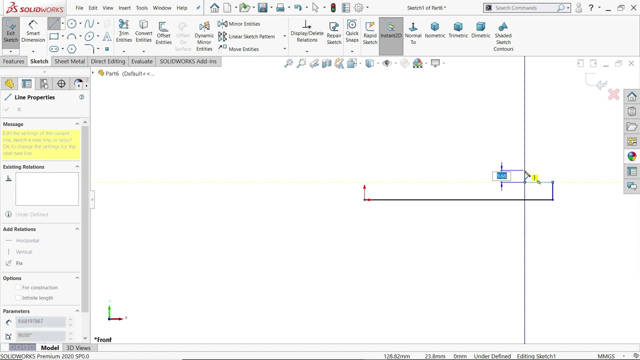 But it's not showing Here. front plane is sketch. now I will activate line tool and I will start from here. Now, here we are going to create many relations. first I will choose these two lines, and here collinear as well as equal. this is important relation. 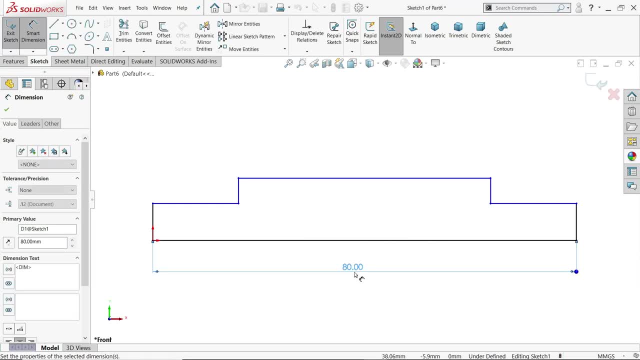 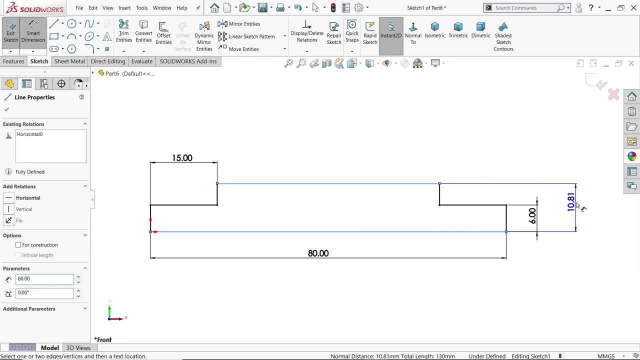 This, All This. Its overall length: 80 millimeter, 50 millimeter, 15 and this one is 50 millimeter. Okay, now, this diameter, It's 12 minutes 6 millimeter. delete this dimension. let make first this dimension 18 by 2. 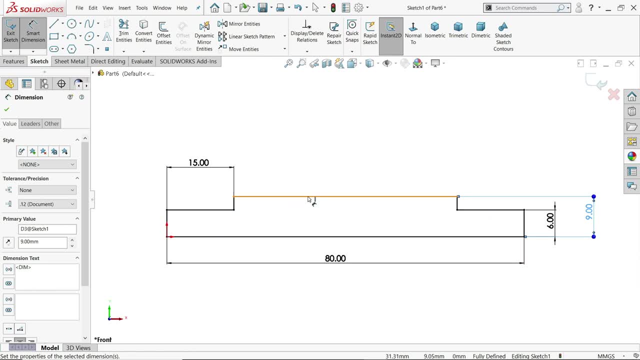 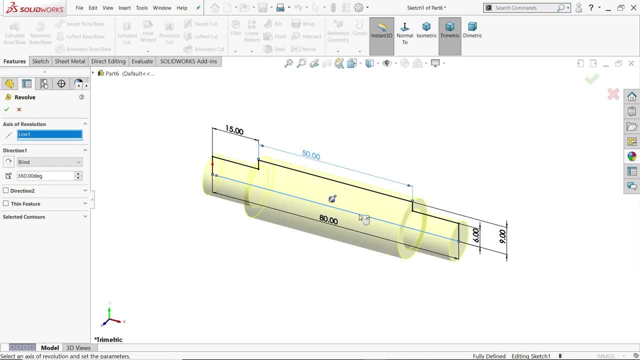 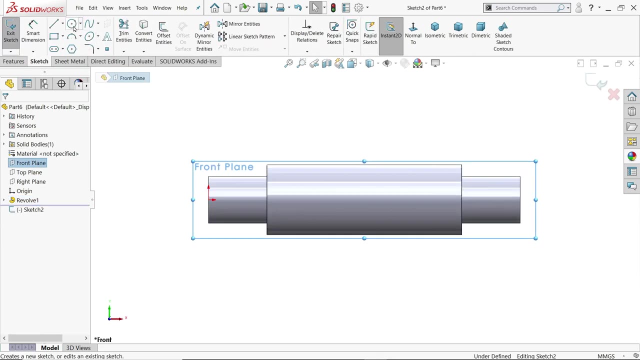 okay, this fully defined, because these two are, if you check this one, 50 by default activate revolve of OS base tool and i'm going to choose this one. say okay again. front plane is sketch. now let me choose here: circle 6 millimeter is smart dimension and 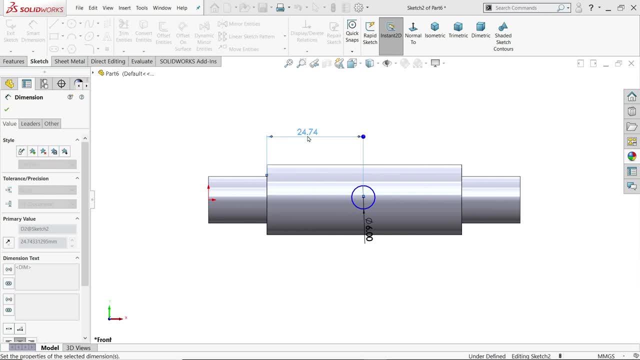 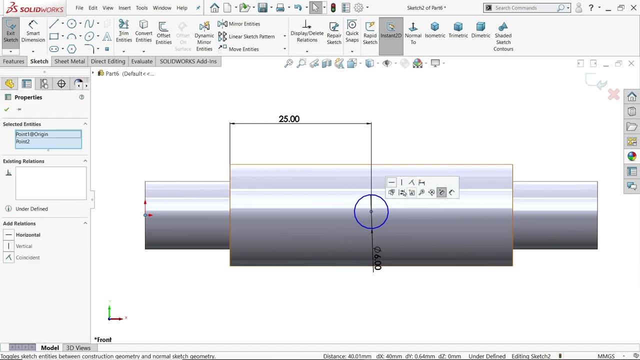 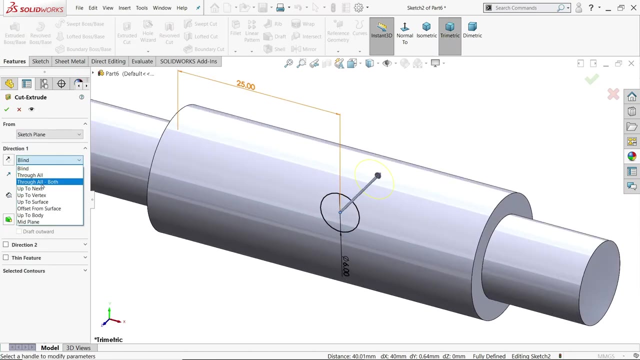 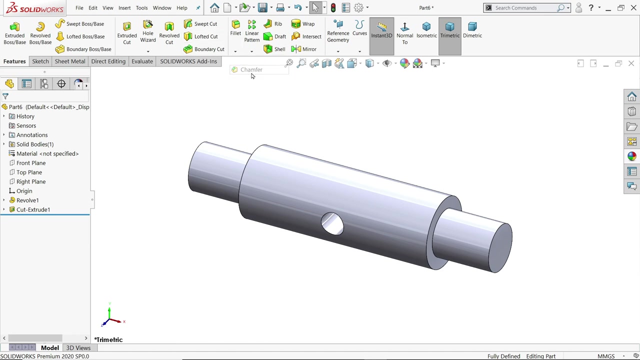 the distance from outer edge is 25. again, we need to create one more relation: hold shift key, select this. two points: horizontal activate extruded cut tool. now here in end condition: choose through all both. say yes, look. activate chamfer angle: chamfer: 1 millimeter and 45 degree. I'll choose both the end age or face both the 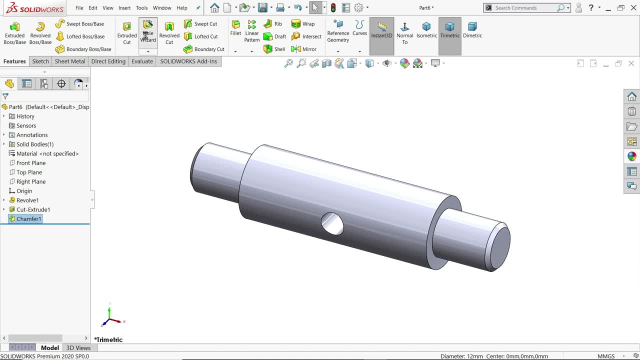 no issue, okay, hole wizard. now we need to create a hole, so I am going to take a hole and here I am going to take drill size. now this is 6 millimeter. okay, now depth is blind and 45 is the depth, and we will keep depth up to. 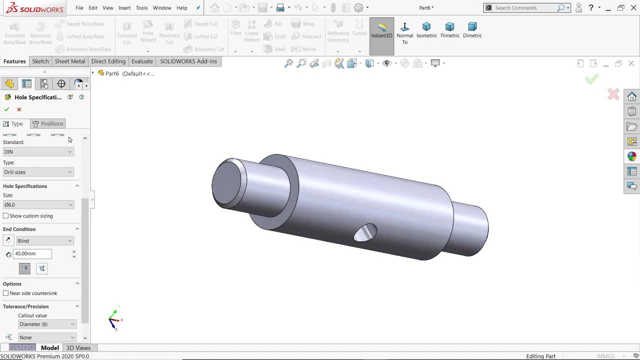 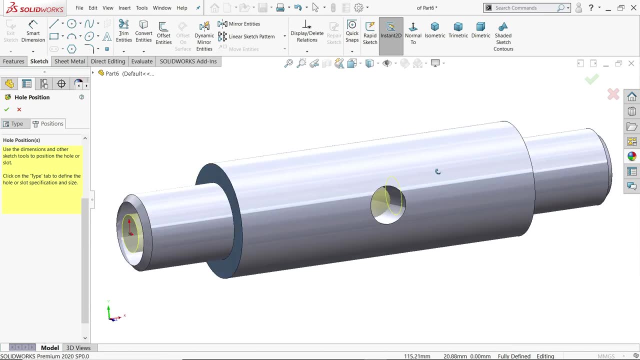 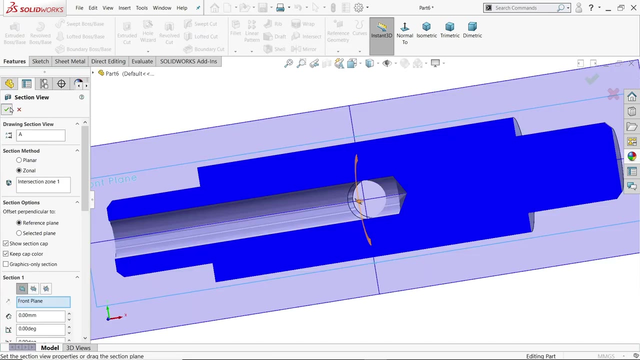 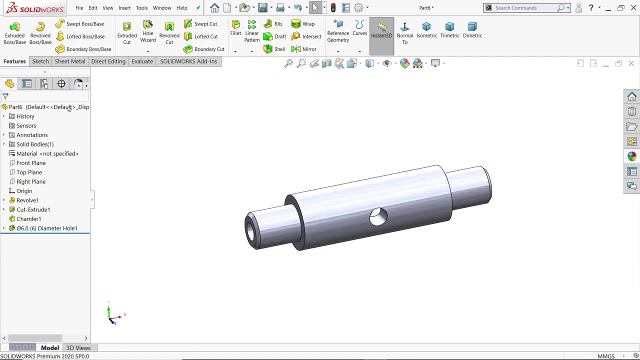 shoulder, not through all position. I'll choose this face and move here, escape key to out and just take the preview. okay, front plane section view. okay, now look, the hole is created. let's add appearance. this is part five: shaft. let's make assembly now here let's start to create. 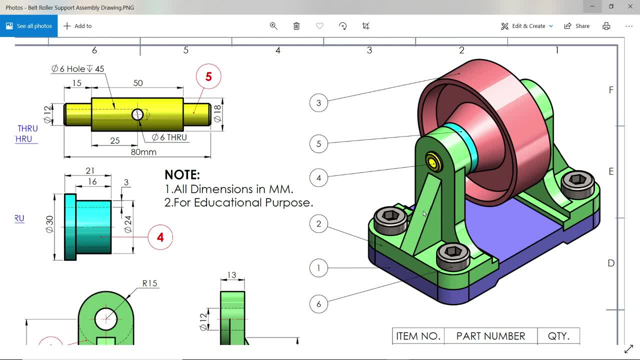 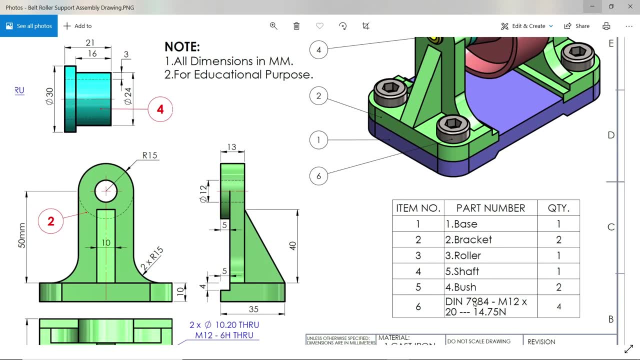 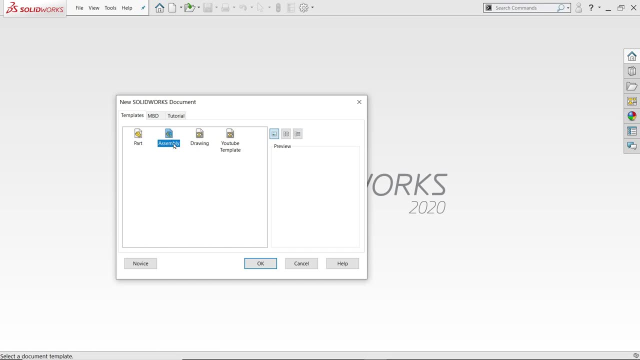 the assembly of belt roller support as an support system. so this is the assembly and here we will add four bolts from system. it is di and seven, nine, eight, four m12 bolt. now open file new and choose your assembly. now open file new and choose your assembly. 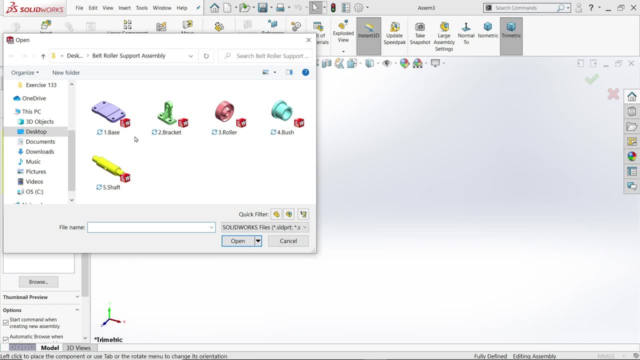 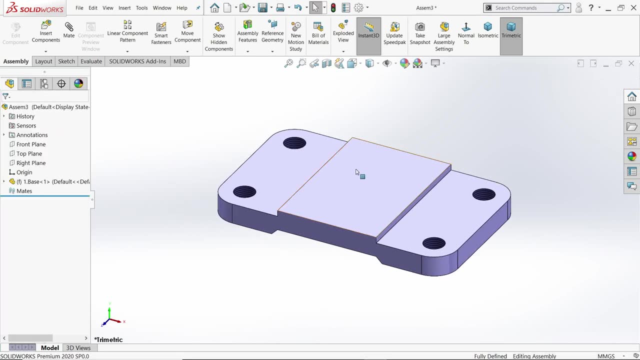 now this is the our window. so first I'll choose base okay, and click somewhere. now, if you are going to check origin point, see right-click float. now choose met. now select both the part of origin points and select connect location. you see the navigation: a heart bar and key bar button one, two, three and point. 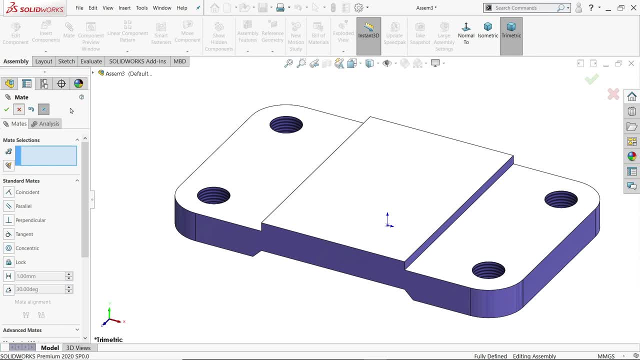 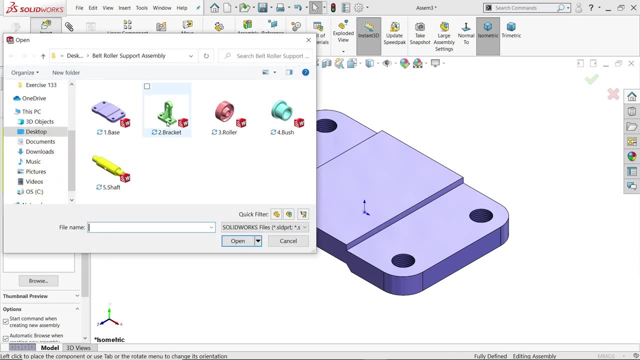 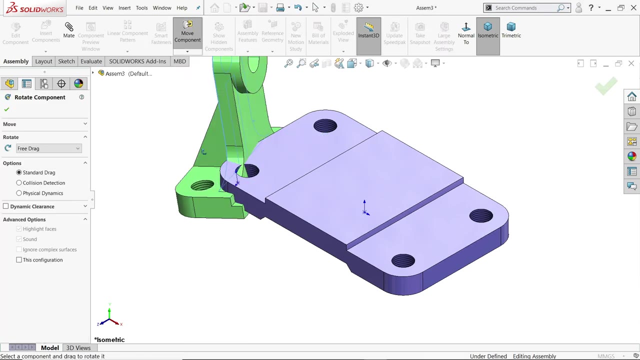 and see it is coincide relation. say ok, cancel. now let's insert another component. now this time i am going to bring bracket. ok, now, here you have option, rotate component, just rotate according to your position. say, ok, now click met. and here i will choose this hole and this. 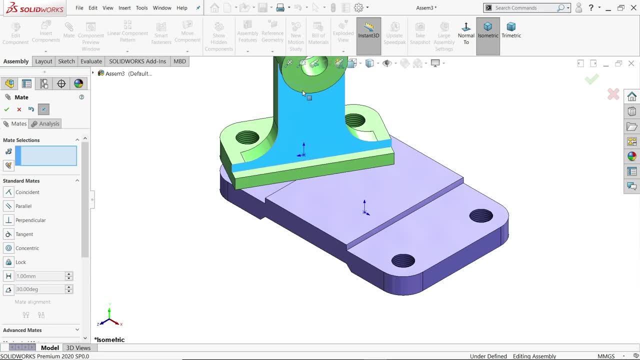 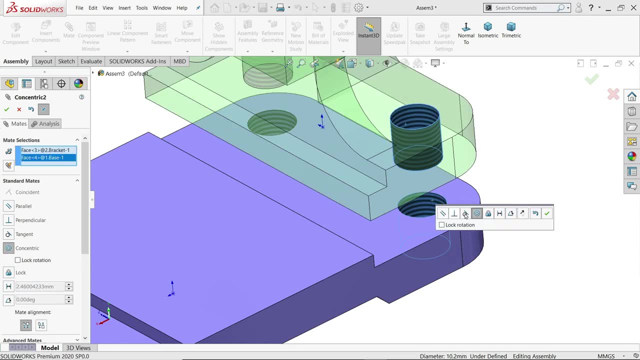 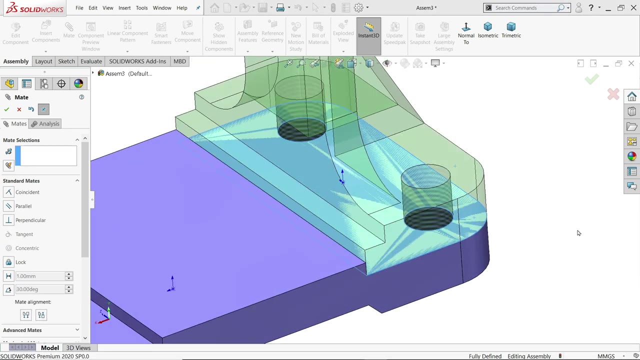 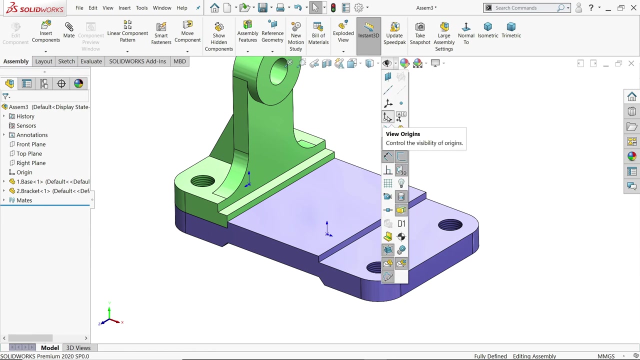 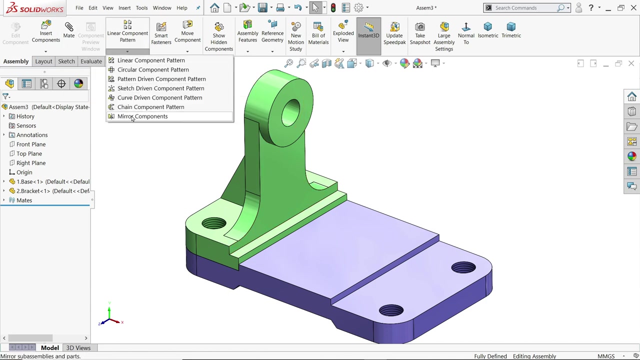 hole, co-centric relation. say yes, just drag somewhere like here i will choose this face, this face, this face. co-centric relation. bottom face and top face coincide relation. see now, just hide origin view. now let's mirror this part. so how we will do? just open mirror component. now here i will choose first plane. so i will choose the plane. 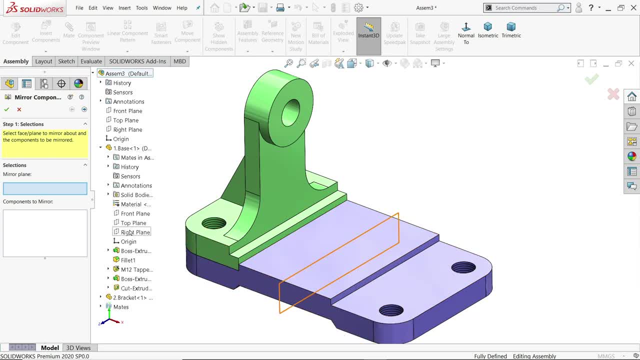 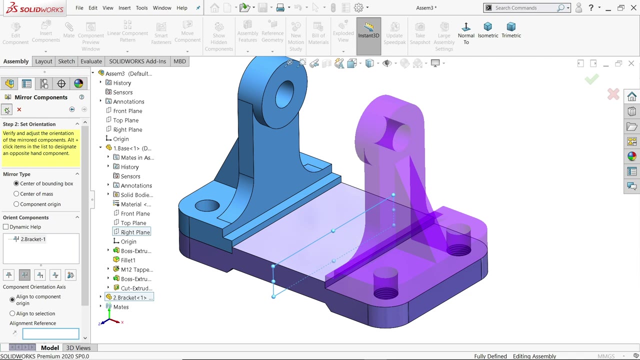 of this part. so just drop down base and you will find here the plane right plane. right plane is the mid plane of this body component. i will choose this one. click here. next you will see the preview. everything keep as it, is, no need to change. say ok, look, it's mirror. 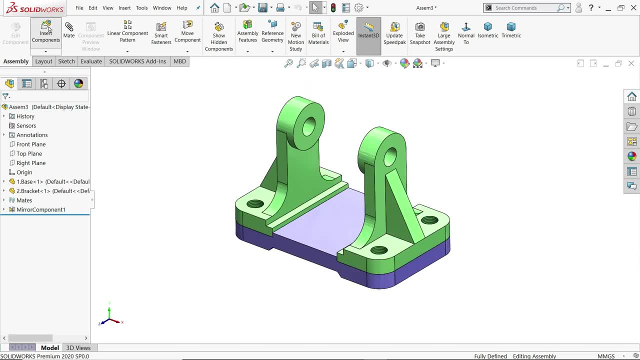 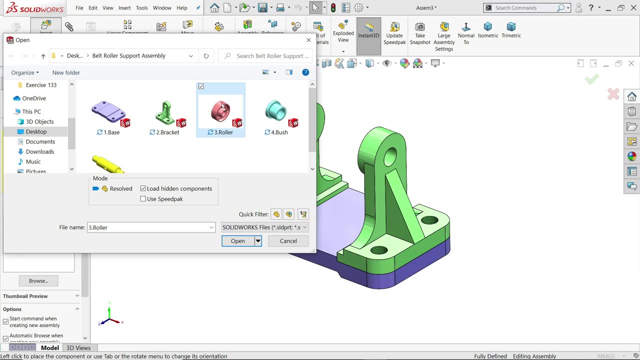 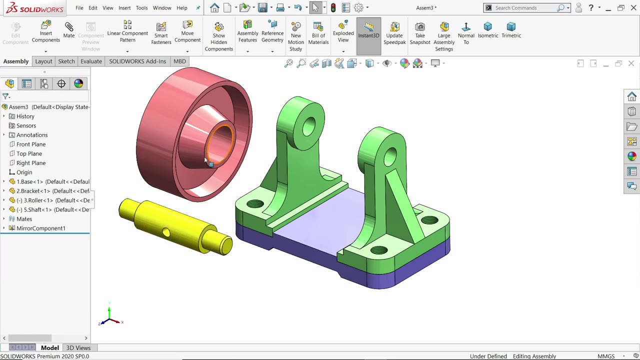 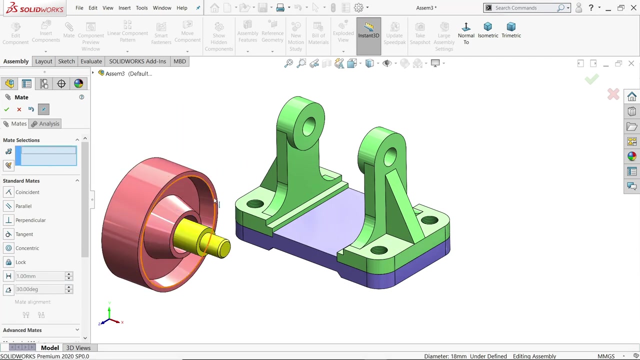 ok, so now i am going to select mirror component now. here i will choose first plane, so i will choose this first plane. well, here i will choose this and i'll also choose this one now. insert component now. this time i will choose one roller and this shaft open. now first make. 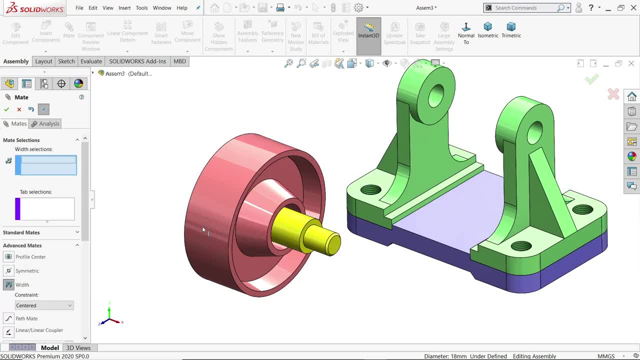 this two relation: keep mat, select this two core centric relation: ok, now, here we will use advanced mat, width mat, i'll choose. ok, this will be the co-centric relation. ok, i'll make it co-centric. okay. and now, here i will use the co-centric and here i will use this: 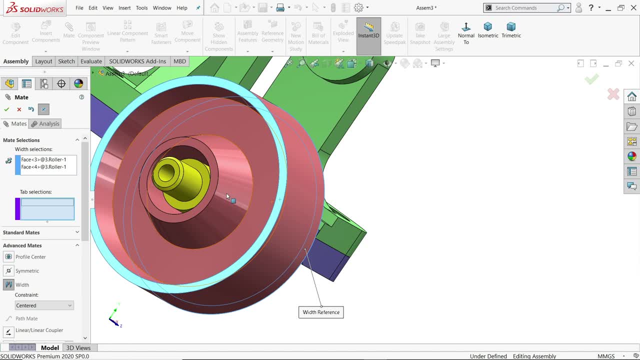 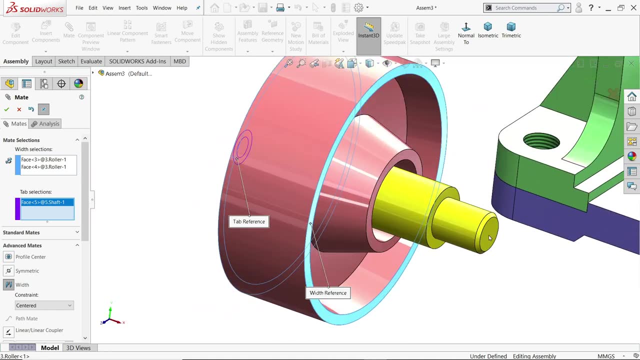 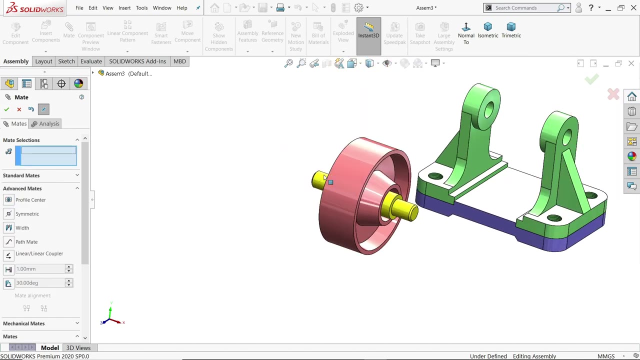 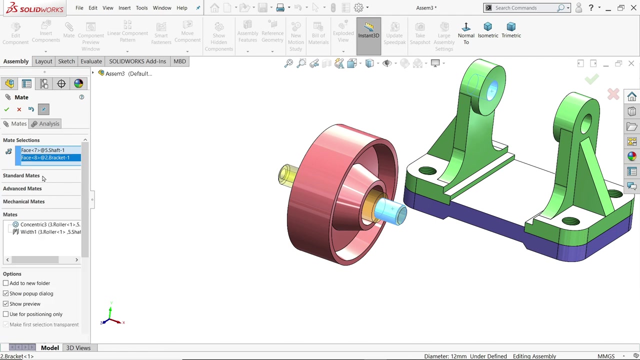 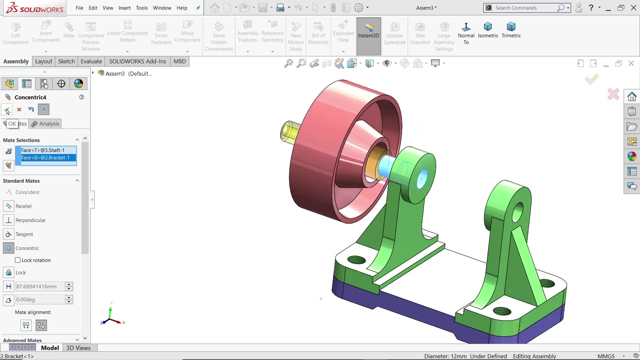 two faces: outer face of this body and outer face of this roller. see here tap section, see this roller going to fix at the center of shaft. say, ok, now this circular face and this circular face keep concentric relation in standard mat. okay, now this one again. we need to apply here: 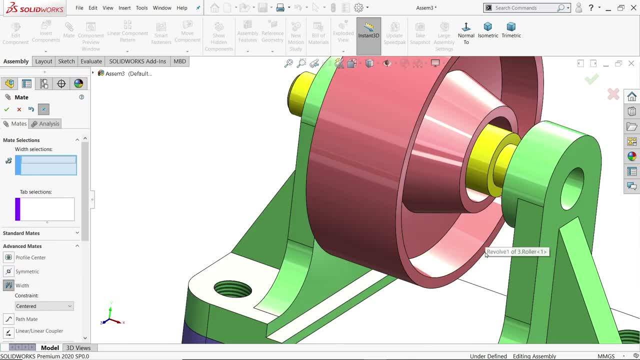 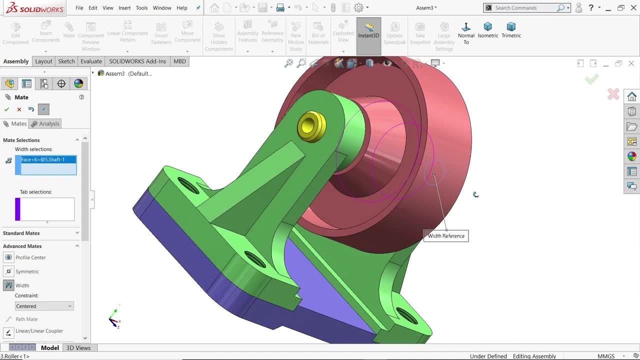 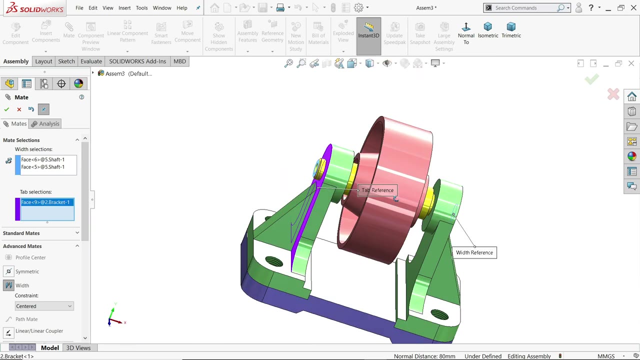 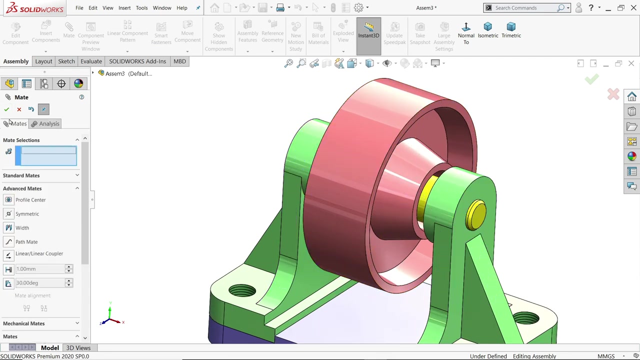 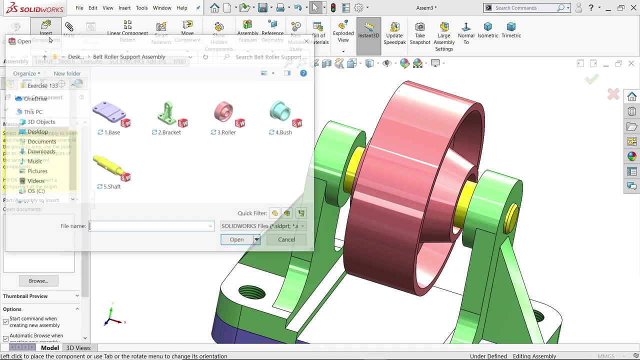 with the mat. this time i'll choose. okay, we are going to apply between these two bodies, so outer part of this roller and outer part of this. okay, this is going to perfectly fix at center. say: okay, now a standard mat. okay, let's bring our last part: insert component bush open. 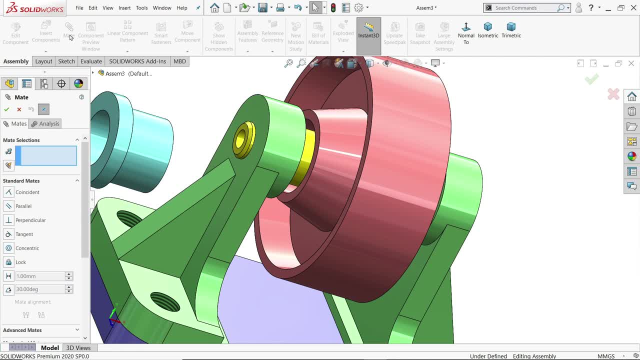 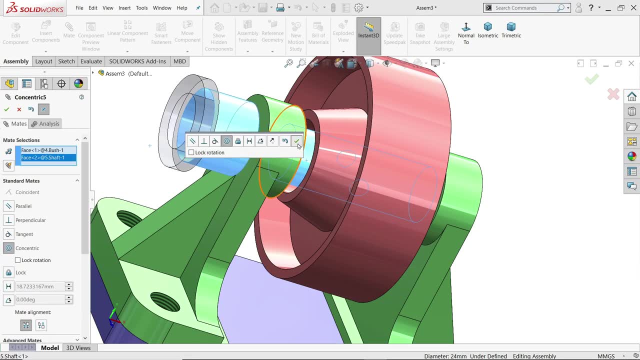 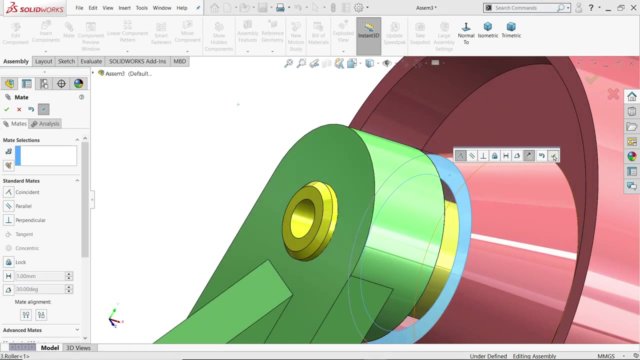 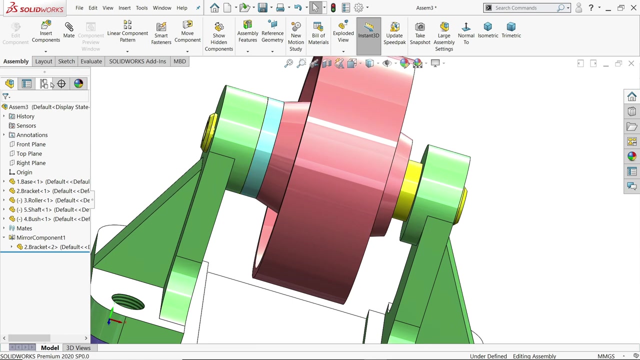 now this is going to fix inside the ruler. select this face and and shaft concentric relation. okay, now select this side wall and this wall, coincident relation. look now this one. we will mirror this component. so mat. oh sorry, let's choose here. drop down linear pattern mirror component. first we have to choose a plane. so plane let's say i'm going to use.